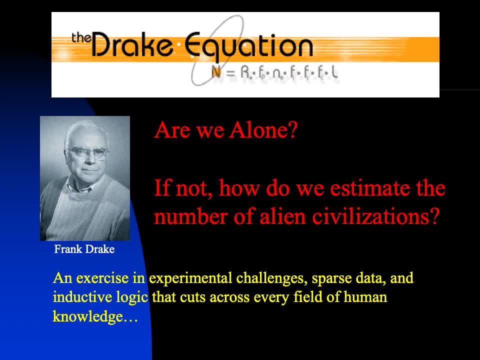 the answer to this question are we alone. So, in other words, he asked himself: how do we estimate what the current number of alien civilizations can be? And one of the beautiful things about this equation is that it's simple, And the second thing is that it really cuts across every field. 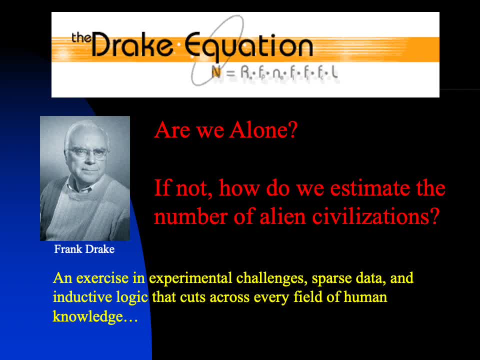 of human knowledge that we actually understand. Some of it is astronomy and some of it is clearly not astronomy. Some of it, of course, is biology and chemistry, And some of it actually has to get into understanding what the current number of alien civilizations can be. And so he asked himself. 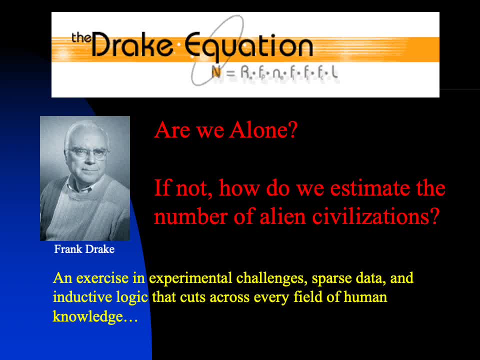 what the economical social consciousness or political social consciousness of these beings might be like, In other words, what their psychology is like. So we'll get into all those questions. It's actually quite interesting And I just want to remind you we live in a very 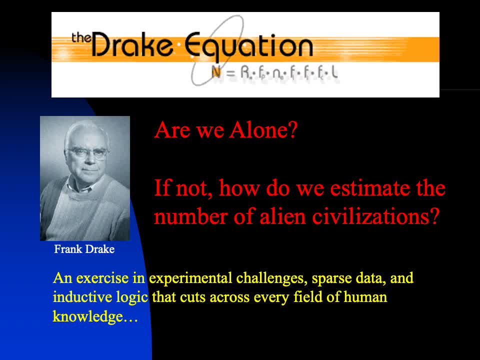 very interesting time, when it's only been a hundred years since we have existed as a civilization that could communicate across the stars, So we are very young in this. Therefore, we don't have a lot of knowledge, And so there's a lot of guesswork that goes into. 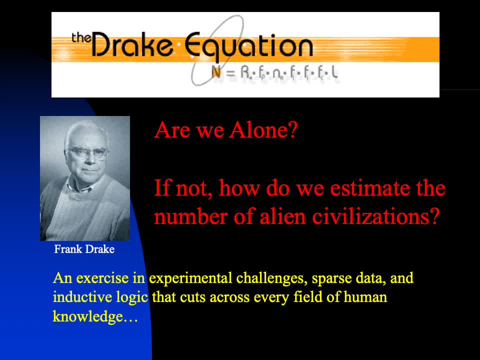 understanding this question. But so far, with all of the observations we've done into space, we've so far not seen any evidence, any observational evidence that there are other technological civilizations out there. But the beautiful thing about science is that every day we learn more and grow, And you'll see as we go through this equation that in fact 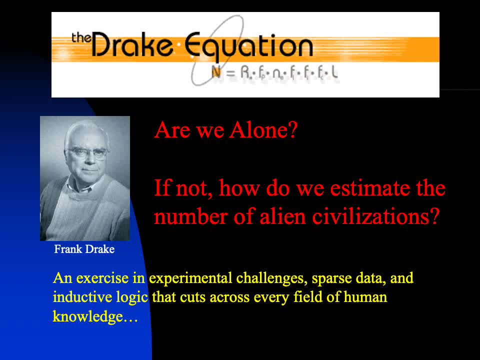 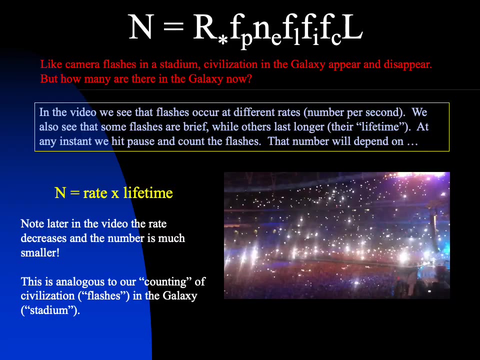 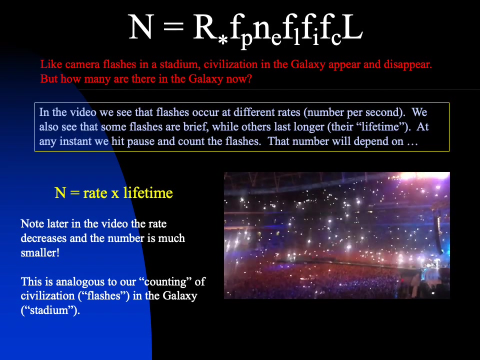 we have learned and grown. We have learned a lot since the day that Frank Drake formulated this question. So, without any further to do, I'm going to take you through a journey of all the terms in the Drake equation. Okay, so the first thing I want to say about civilizations in the galaxy is that they come. 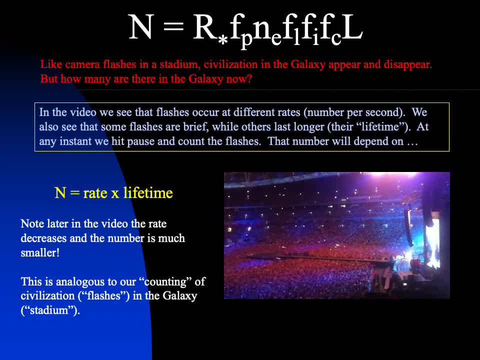 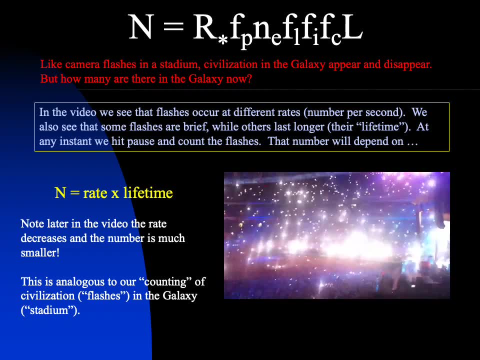 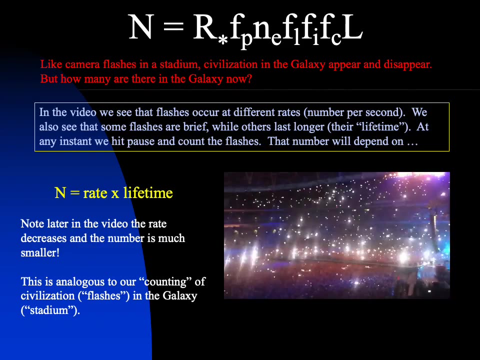 and go- At least we expect them to come and go, So they might evolve into existence, stay in a communicative phase for a period of time and then disappear. And when I say communicative, I mean the ability to communicate across the distances of the stars. And I'd like 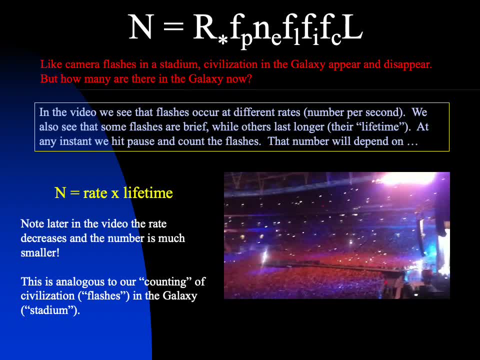 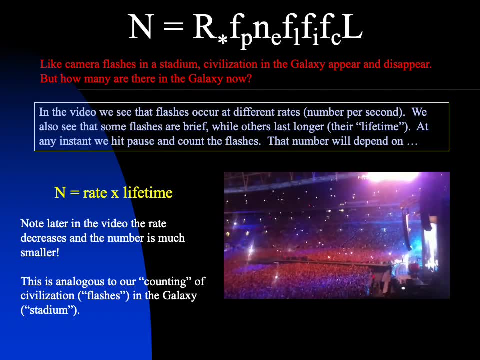 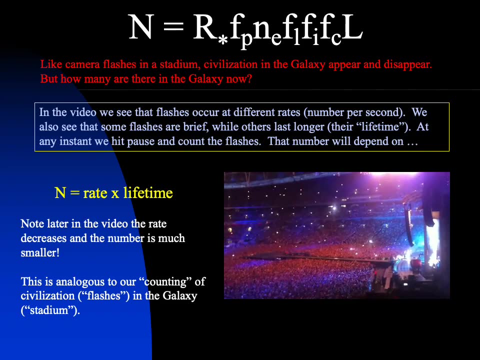 to liken this to flashes in, say, a soccer match or a football stadium during halftime- camera flashes. Camera flashes come and go. Some are very rapid and some are very long, And if you will watch this video here for a brief second, you'll see that some flashes occur. 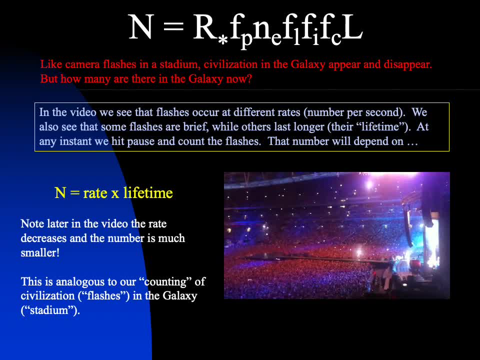 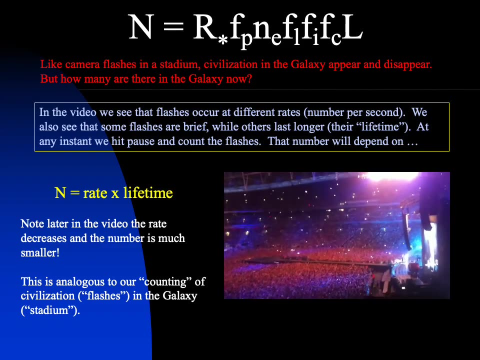 very rapidly and some are very long, And what happens is that if you pause the video any given time and count the flashes, okay, what you will be seeing there is that number that you count will be dependent upon two things. It will be dependent upon the rate at which new camera 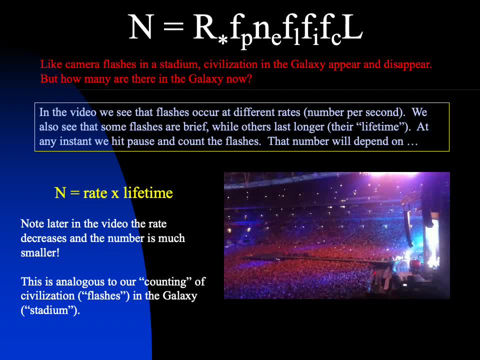 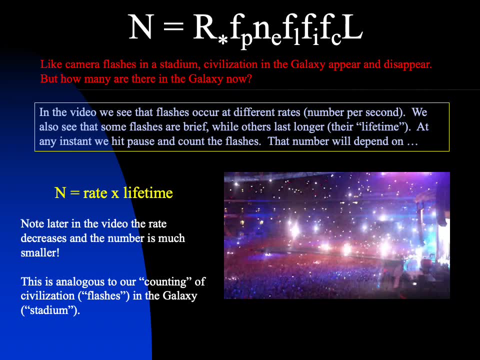 of flashes are coming into existence. multiplied by the average lifetime of a flash, Say, there's 10 flashes coming in every second and each flash lasts about one second. Then you multiply those together and you get. when you hit the pause button, you should see about 10 flashes, no matter. 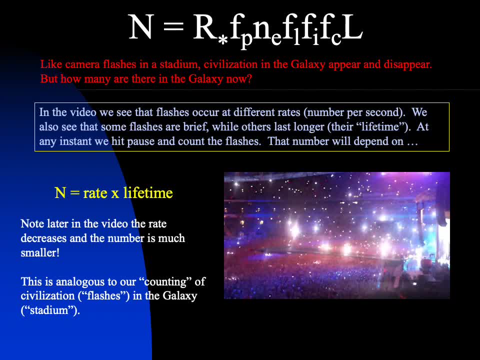 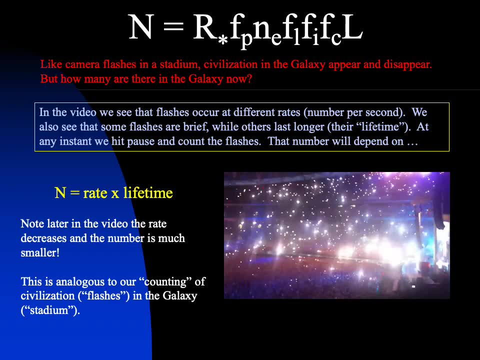 when you hit the pause button. As you can see in the beginning of the video, the number of flashes that are coming into existence is a very high rate, and later in the video the rate is very low. But you can also see- and I want you to watch this one more time- some of these flashes sustained for 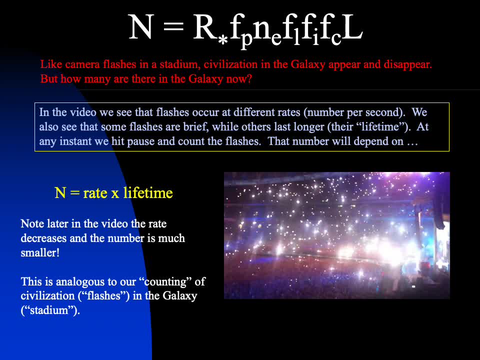 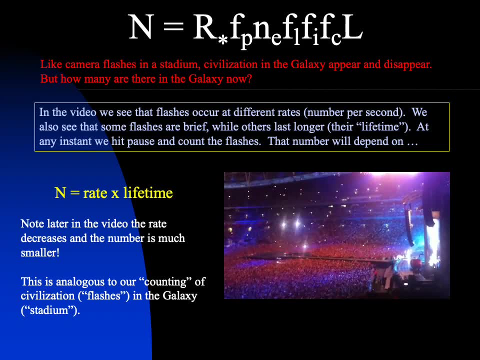 a long period of time, almost throughout the entire video, whereas some of them come and go rapidly. So let me watch that sometime. now. You can see some flashes have actually persisted for a long time. The point is, if you hit pause at any point in time, that number at that moment will be the rate of new. 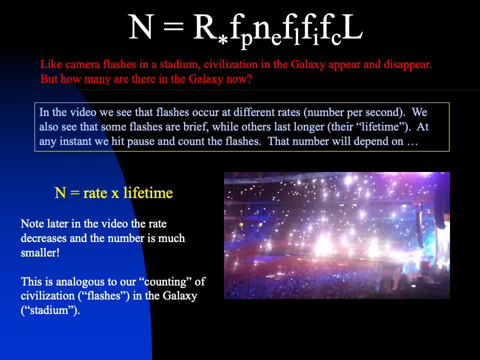 flashes times the average lifetime of a flash, And so that is the logic behind the Drake equation. You can think of a new civilization, a new technological civilization that could communicate across the stars, coming into existence, and there would be a rate at which new ones are coming into existence in the galaxy And then they stick around for a 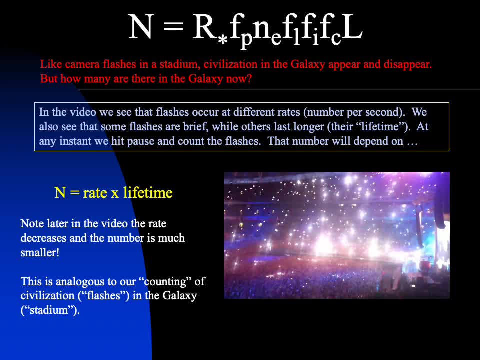 certain amount of time, their average lifetime, that they're communicative across stellar distances, And if we can figure out the rate of new ones coming into existence in the galaxy and the average lifetime of civilizations, we can simply multiply those two numbers together and get in the total number of civilizations that we should see at any moment. 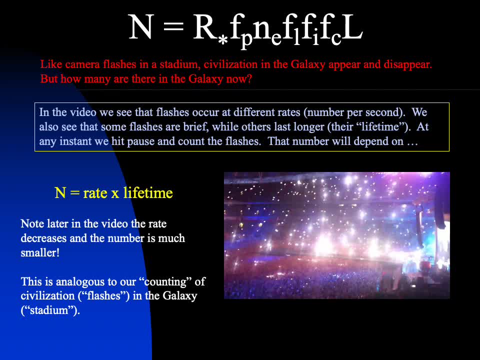 when we hit the pause button on what's going on in the galaxy. Of course, the galaxy, our sun is about four and a half billion years old and the galaxy is about 10 billion years old, So our current lifetime is effectively the same. 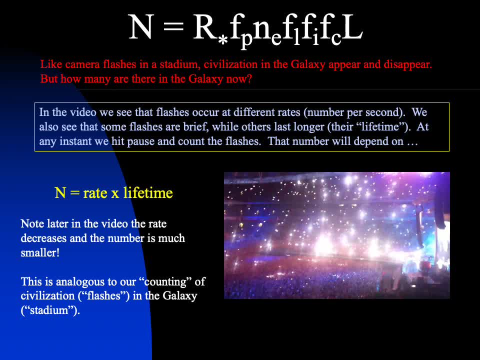 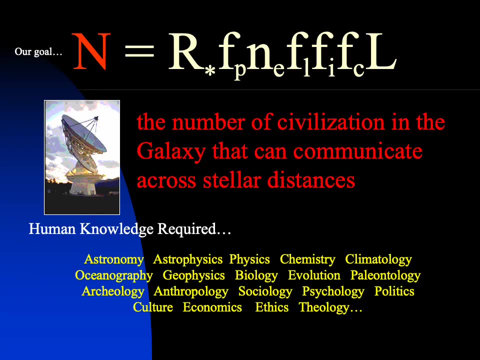 so short that it's like having the pause button set at now at t equals 10 billion years in the galaxy. So that's the way that we view the Drake equation. Our goal is to calculate n, the number of civilizations in the galaxy that can communicate across stellar distances. 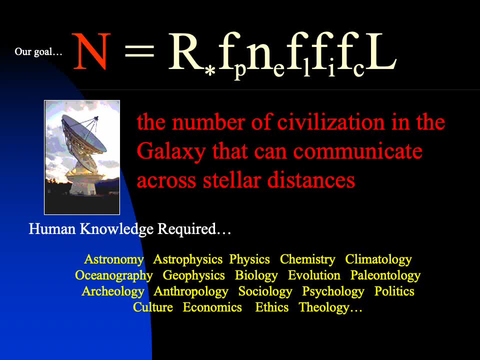 Atop the slide is the Drake equation itself, which you've been seeing in the last few slides. I've highlighted n in orange or red, and so when you see a variable in the equation highlighted in red, that's to remind you that that's the variable that we'll be talking about, And so we're going to start. 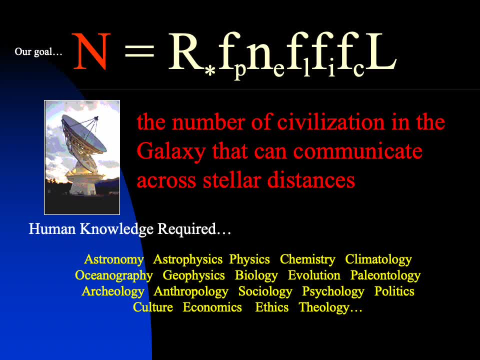 with n. It's on the left hand side of the equation. That's the number we wish to estimate or calculate, And that number is defined as the number of civilizations in the galaxy- our galaxy, not the universe in our galaxy- that can communicate across stellar distances. 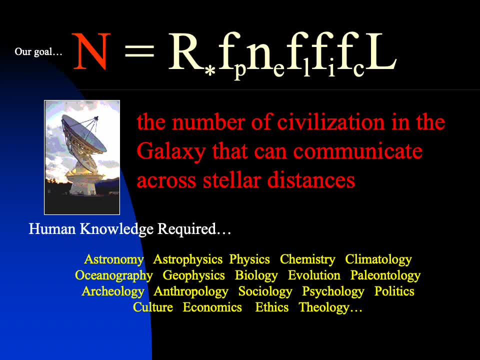 As we travel down this equation. it equals r sub star f sub p times n sub e times f sub l times f sub i times f sub c times l. We are going to talk about astronomy, astrophysics, physics, chemistry, climatology, oceanography, geophysics, biology, evolution, paleontology, archaeology, anthropology. 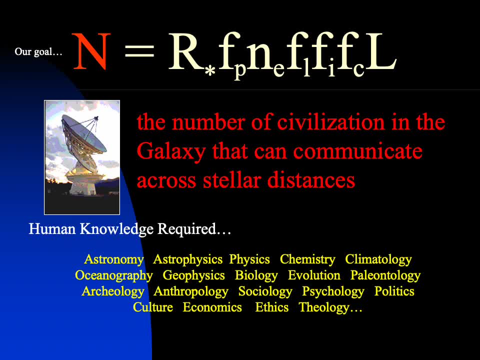 sociology, physiology, politics, culture, economics, ethics, and a little bit even you could touch on theology. The point is, as we go down this equation, we are basically going to go down this chain of human knowledge, And as we explore this, we'll find out that in some cases, for some 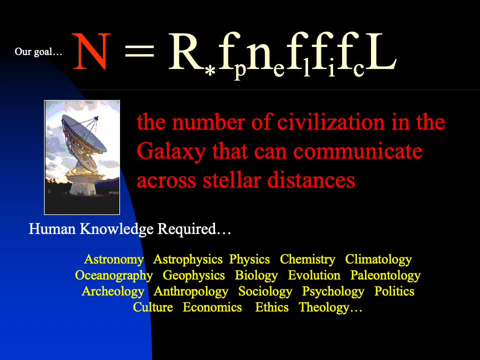 of these terms in the equation. we only have our existence or the existence of life on earth in order to make any estimates. So that makes understanding, estimating the Drake equation quite difficult in some cases. So we have to really study our own existence, our own evolution, our own. 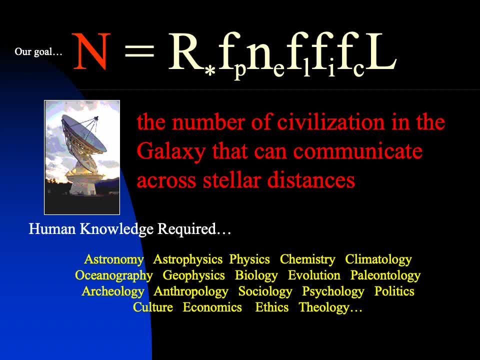 psychology in order to understand or try to see ourselves in some kind of context for which we have no other data. So I'm going to continue to define these terms, but first I want to re-emphasize for you, in the next slide, the concept of rate times. time: Rate of new civilizations, times the average lifetime will be. 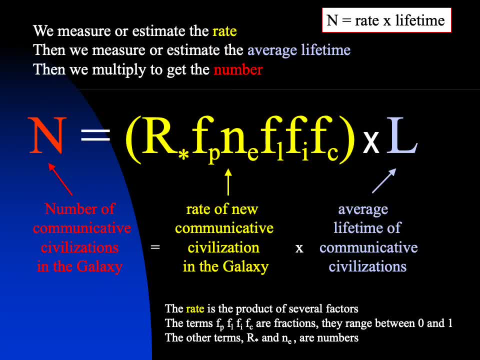 what gives us this number? Now, in the upper right hand corner, I have the simple equation that n equals rate times lifetime, and that, effectively, is the simple version of the Drake equation. Like I said before, with the flashes in the football stadium, if we can estimate the rate, 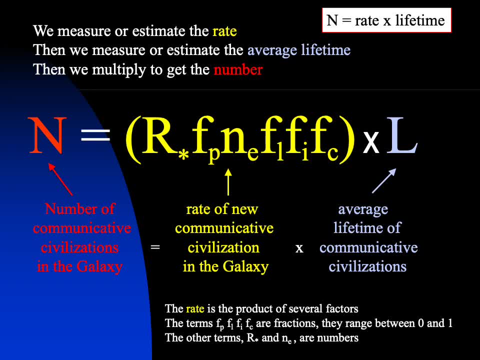 and we can measure the average lifetime, knowing that some of the flashes are short and some of the flashes can be long. We take that average and we multiply that together with the rate, we get the number. And so I've drawn the Drake equation here, with, in a sense, as an n equals rate, times. 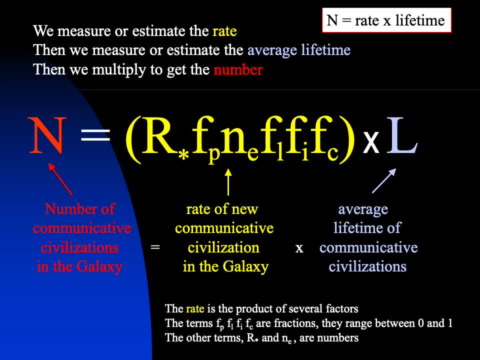 lifetime simplified version. One of the reasons we have the little phenomenon here of motorcycle to push萬 version On the left in red- is the number of communicative civilizations in the galaxy, and that's equal to- and you can see it in words here- the rate of new communicative civilizations. 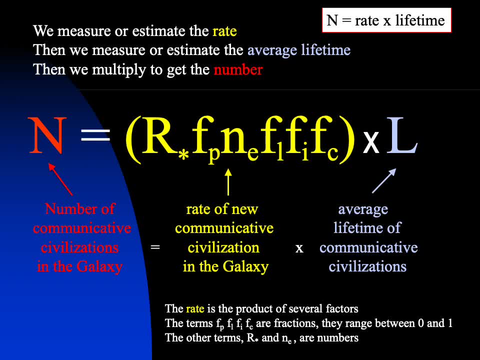 in the galaxy times the average lifetime of communicative civilizations. Now it turns out that if we just talk about the average lifetime first, that's just a simple single variable that we label L okay, and we put in the number for whatever the average lifetime is for that variable. 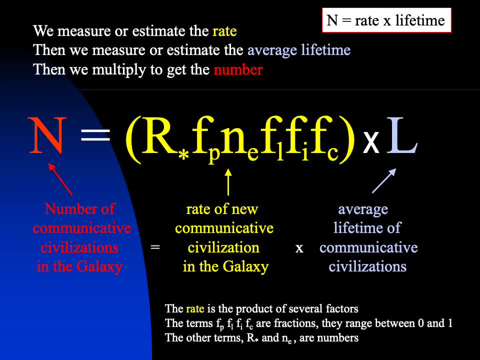 But the rate for communicative civilizations, on the other hand, is a complex product of several terms, and we're going to go through each one of these terms step by step. What I want you to understand about this equation is that whenever you see an F, that represents 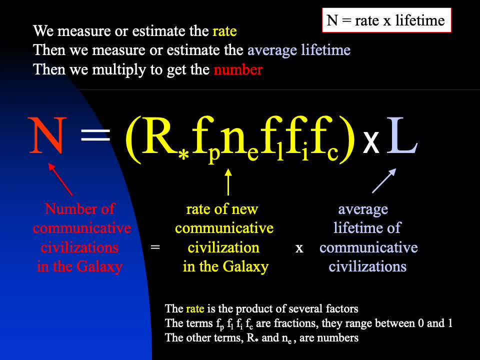 a fraction, That means it represents a number that ranges between zero and one, say a half or 0.9 or something like that. So that's basically telling us about some kind of fractional number, not a number itself. However, the terms r, star and m sub e- those are numbers. 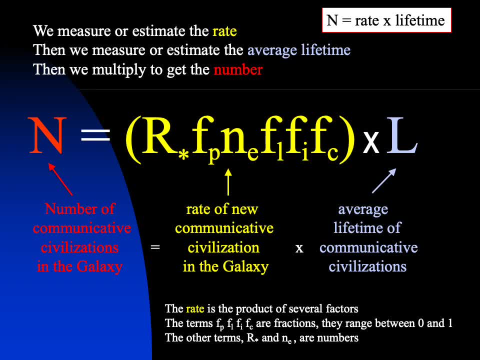 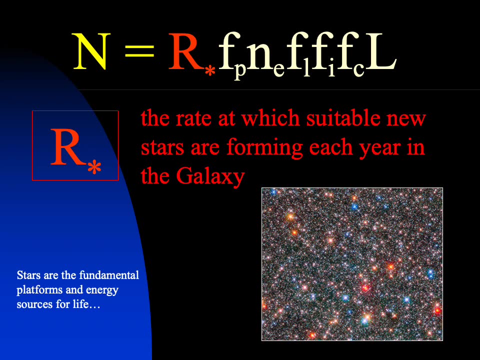 and so those can be actually any number that we know about. Some of them can be, it could be much greater than one, but the Fs, those are fractions, and they will always range between zero and one, The first term that actually helps us estimate the rate of new civilizations in the galaxy. 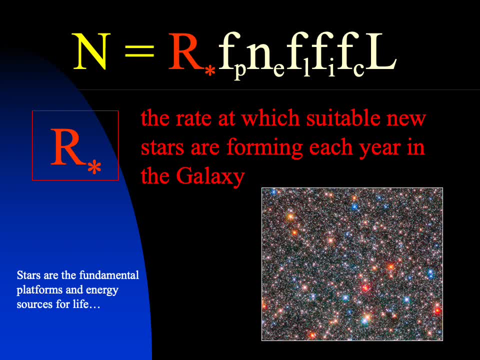 is r star, So we believe that stars are the fundamental platforms of energy for the sources of life. If you think about being in deep space, there's not a lot of energy and the most important thing is that you need an energy gradient. You need energy gradients of energy. 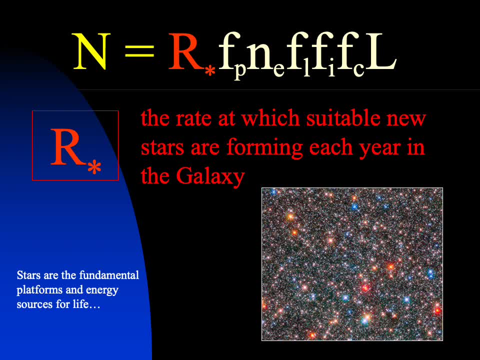 that changes from one place to the other for life to then be able to draw from that energy, because it's the transfer of energy from one form to the other or one location to another that provides ability for metabolism to move forward. so you need areas where there's differences in energy. 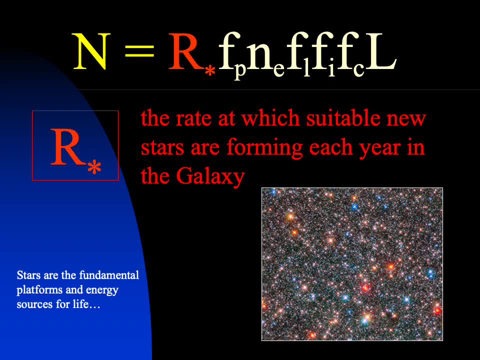 and so we believe that around stars is one of the best candidate places, if not really, for our understanding of the stability of biochemistry, the only platform. however, we must keep an open mind but thinking of the 1960s and whatnot, definitely putting life around a. 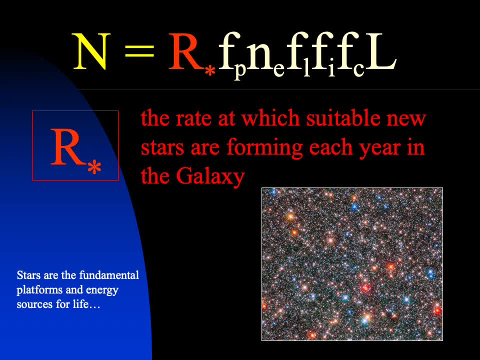 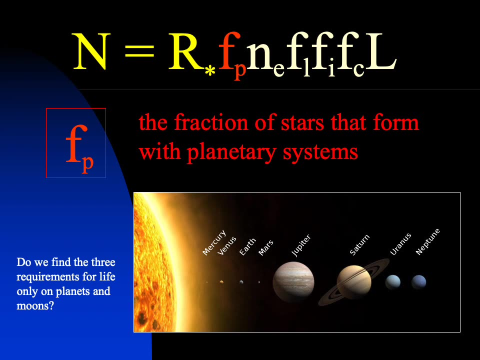 central star was the conventional wisdom. it remains pretty much the conventional wisdom today. so our first term is our star and that is the rate at which suitable and new stars are forming each day in the galaxy. now we also think that, as far as finding locations that would satisfy the three requirements for life, 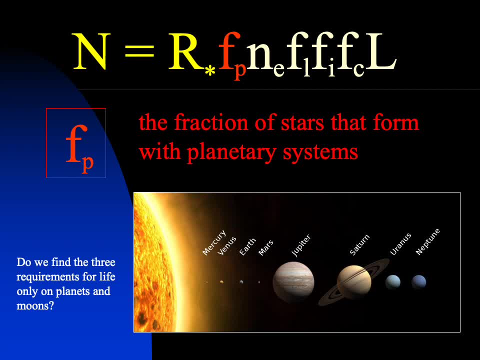 which, if we recall from our previous lecture, is energy source. number two would be the chemical elements required for life, and the third one would be a transport medium, a liquid transport medium for metabolism for which water was consumed, and the third one would be a transport medium for metabolism for which water was consumed, and the third one would be a transport medium for. 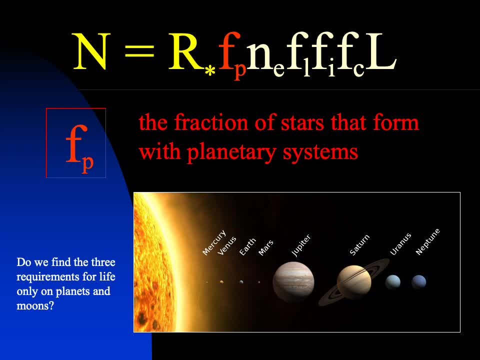 which I have considered so far to be the best candidate. now it would seem logical that planets that are locations which really concentrate these three requirements for life. and so the next thing, thinkers that does considered so far to be the best candidate. now it would seem logical that planets 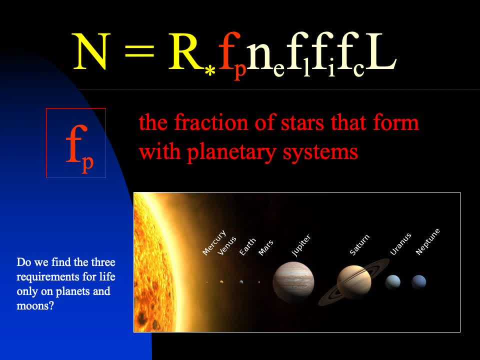 and so the next thing we want to know is well, of all these new stars that come into existence every year in the galaxy, we want to know is well, of all these new stars that come into existence every year in the galaxy, we would want to know what fraction of them form planetary systems around them. 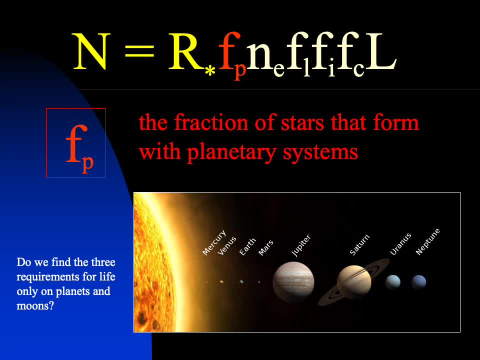 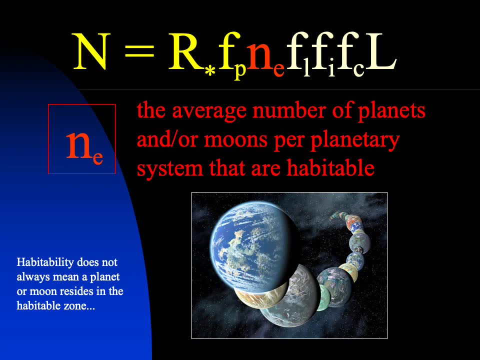 So our next term here is F sub p, the fraction of stars that form with planetary systems. So, moving along to the next term, it's N sub e, and this is a number. This is an average number, and what we want to know now is: in these new stars that form? 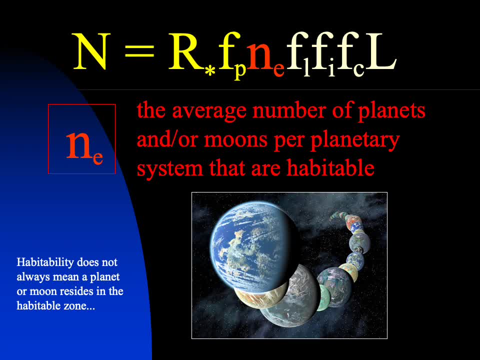 every year that have planetary systems form around them. what's the average number of planets or moons in the systems that are actually habitable? So remember that habitability doesn't always mean that a planet or moon resides in a habitable zone, and I remind you that the habitable zone is the shell around a star that have 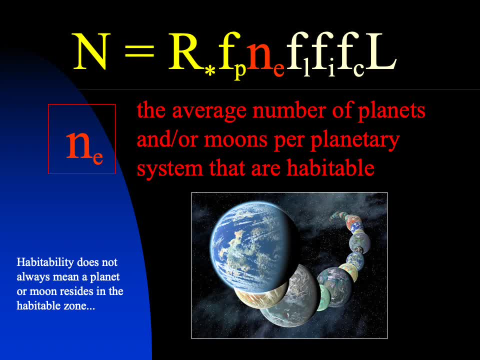 an inner distance and an outer distance For which, if you put a terrestrial-like planet in that region, that distance from the star, liquid water could survive on the surface, And so Earth clearly is in the Sun's habitable zone. But there are, as we've seen through our other studies, the moons around Jupiter, the Jovian, 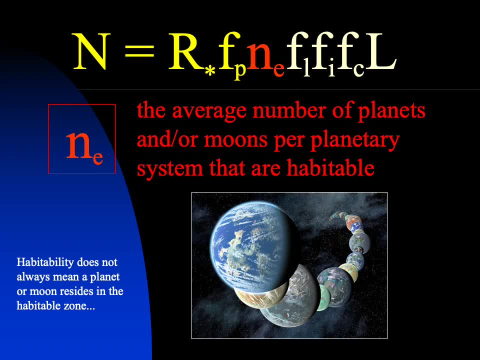 moons around Jupiter, particularly Europa, which has underground water. We have around Saturn Encephalus, which has water geysers, And so it's very possible that some moons around other planets could also be in a sense habitable according to having the three criteria for life that we discussed. 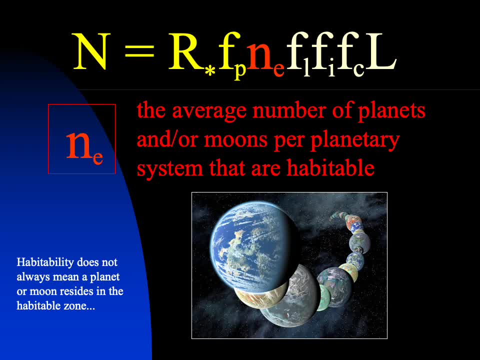 So you need to keep an open mind about how to count, whether it's planets or moons. But in the end, once you have planetary systems form, you would like to know what's the average number of planets or moons per planetary system that are actually habitable. 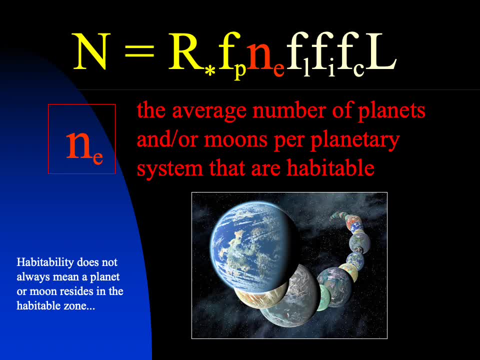 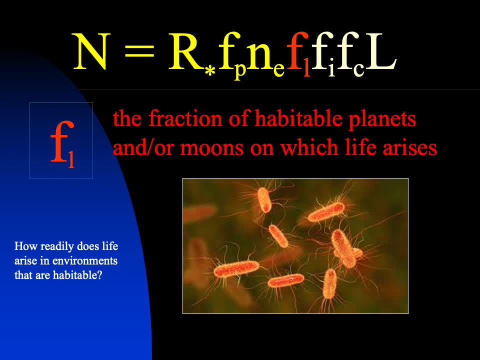 So that's what we're going to talk about today And that would be couched in the term n sub e. Now, once we have an estimate for the number of planets that are, say, habitable, we come up with this product that's in yellow. here r star times f sub p. times n sub e. 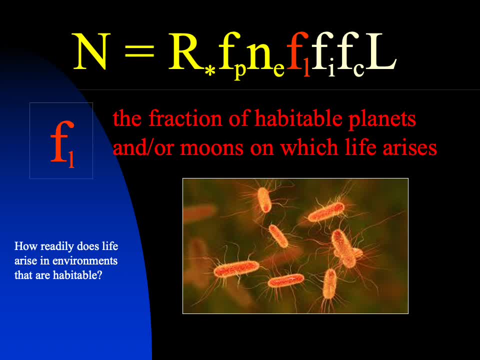 Then we want to know on what fraction of these habitable worlds would life actually arise? And so this is the term f sub l. Again, it's a fraction between zero and one, And really this fraction is addressing the simple question: how readily does life arise? 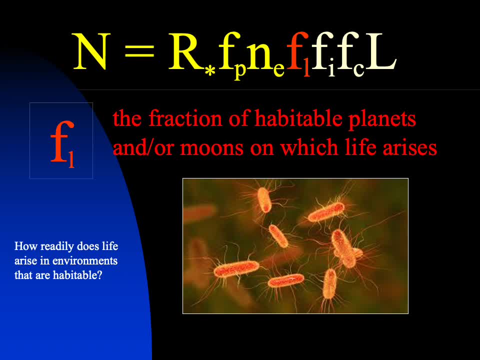 in environments that are habitable in our galaxy? We don't know the answer to that question. All we really have is the Earth to go based on, to be based on, And this is one of the reasons why finding life on one of the other bodies in our galaxy. 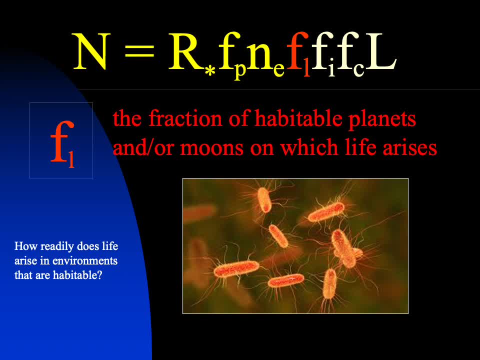 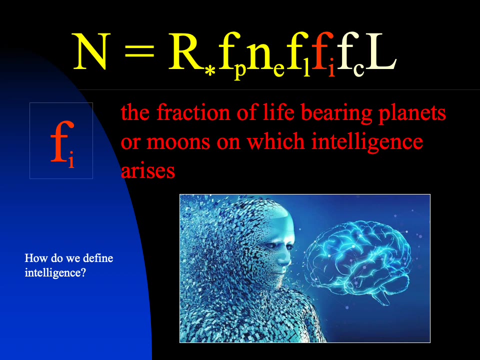 in our solar system is so important. So this is the term for life: the fraction of habitable planets and or moons in which life arises, f sub l. The next term in the Drake equation is f sub i. So once we have some indication of what fraction of these Earth-like, or I should say, habitable, 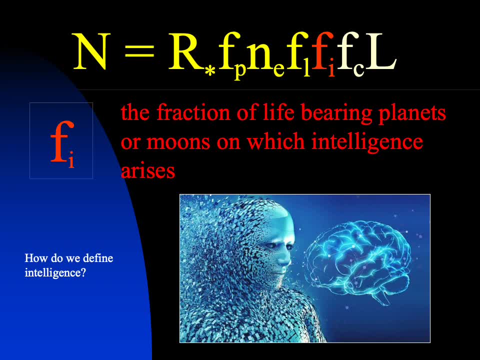 planets that come into existence In the galaxy every year. we want to know on what fraction of the life-bearing planets actually will have an intelligent species arise Now. this fraction involves our trying to understand the record of Earth and the record of how intelligence has developed as a Darwinian strategy for survival of a species. 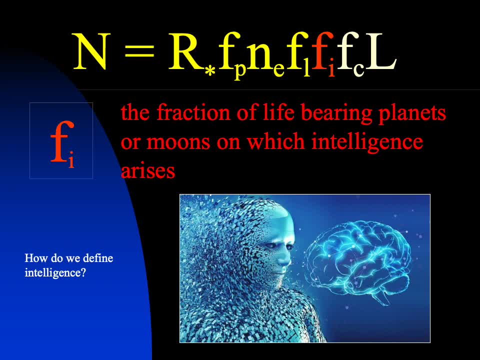 There's a lot to be learned about that. We're really doing well in learning a lot about that. Research has been moving forward, but nonetheless it's an area that is nascent as far as research goes. Now- one of the hardest parts about this, in the same way that we have to have a clear 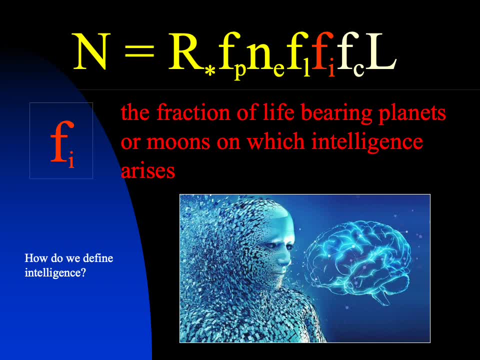 definition of life, which of course, we did earlier in the class. we have to have a clear definition for what is intelligence, which we haven't yet done in this class. so some point today's life. In this lecture, I will talk about how we define intelligence in a simple way. it has. 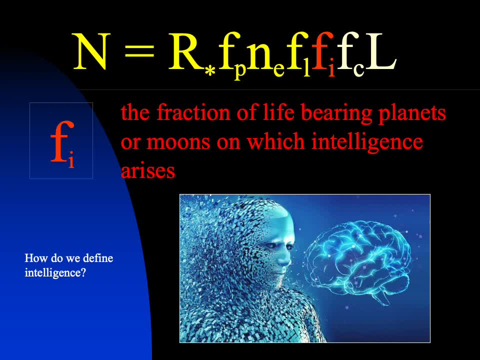 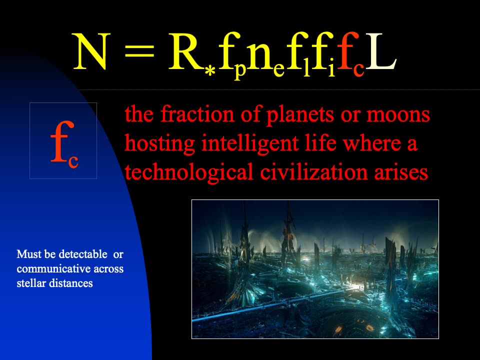 its limits, but in a simple way to help us address this question. So F sub i: the fraction of life-bearing planets or moons on which intelligence arises. Now knowing something about the number of intelligent species that arise in the galaxy every year, or the rate at which they do when you multiply r star times, F sub p times. 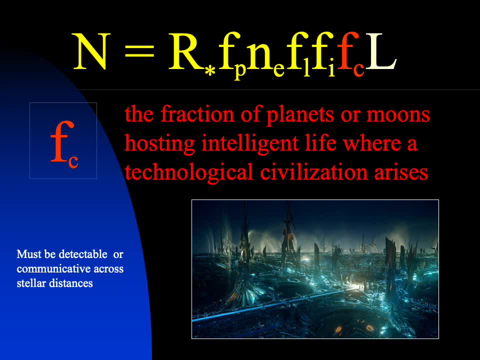 N sub e, f sub l times, f sub i. That gives you the rate of new intelligent species arising in the galaxy. Now we want to see through the next filter, which is: do they develop into a technological civilizations like we did? Okay, so to to meet the criteria of our drake equation, we have to 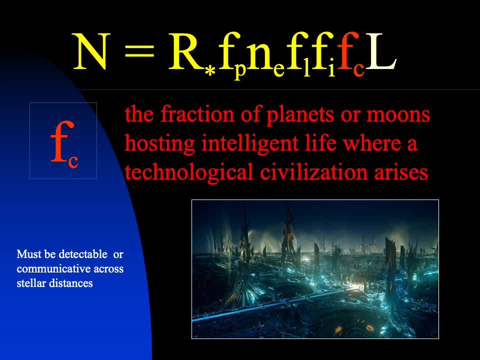 have a detectable or communicative civilization that can do that across stellar distances. So we come up with the next fraction, the fraction of planets or moons that host intelligent life, where a technological civilization will arise. Now we only have one data point for that, That's us. 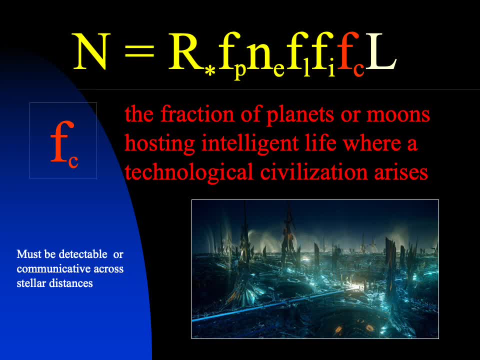 Okay now, as we're going to talk about other intelligent beings exist on this planet, and other very intelligent beings exist on this planet. So all of these intelligent beings have existed in in the past, but they did not develop technological civilizations. So what was different? What variables may have been important for the transition from intelligence? 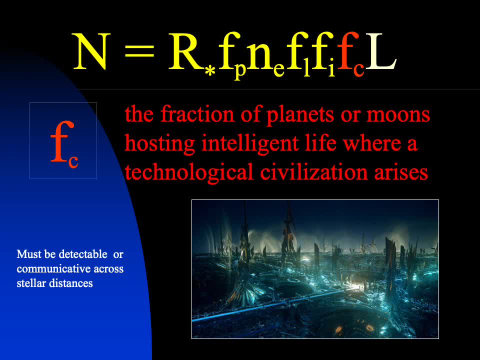 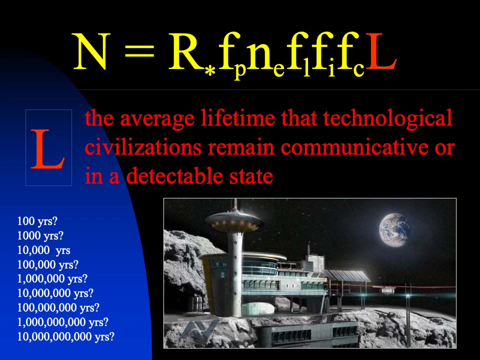 to blossoming into technology. So f sub c, the fraction of planets or moons hosting intelligent life where a technological civilization arises. Okay, so you can see there in yellow r star: times f sub p, times n sub e, times f sub l, times f sub i, times f sub c. 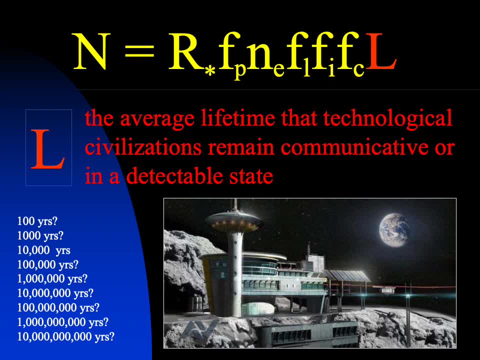 That product gives you the rate at which new technological civilizations are coming into existence in the galaxy every year. And now we need to multiply that by l, the average lifetime that technological civilizations will remain in the communicative or detectable state. Now you can be a technological civilization, but not necessarily communicate across the stars. 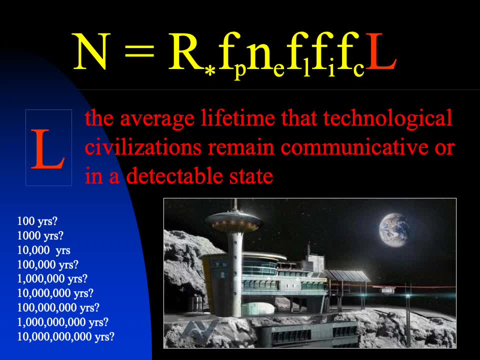 You might baffle your technology so that it becomes silent. We'll talk about that, And that comes down to the psychology of the intelligent beings, or the civilization. The question really is: how long is this? 100 years, 1,000 years, 10,000,, et cetera, et cetera, up to 10 billion years. 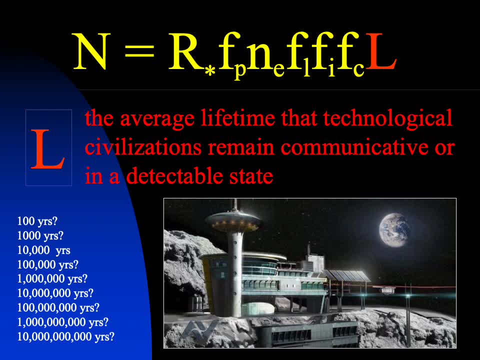 In other words, a civilization that, once it came into existence, would exist for the entire length of the known age of the galaxy. Now I want to remind you that we're talking about the average lifetime. Some civilizations may Only last a hundred years. 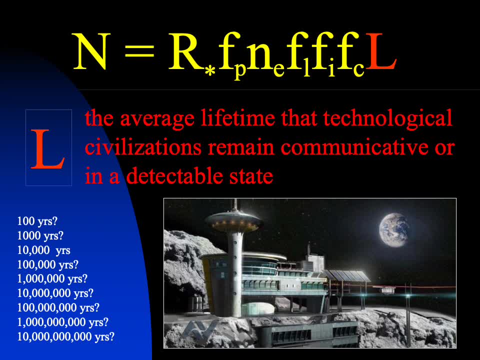 Others may last a hundred million years. We need to know the relative numbers of how many live short lives and how many live long lives, And if we know the relative numbers of all that distribution of possible technological Civilization lifetimes, we can then calculate the average. 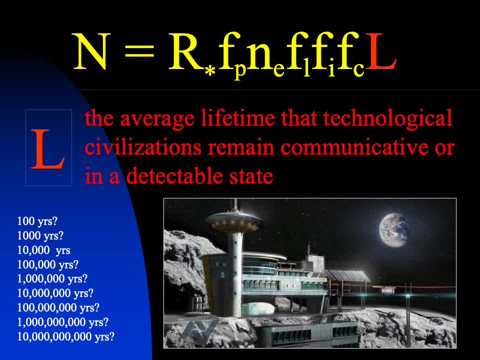 Now we clearly have no clue About the typical lifetime or the distribution of lifetimes of technological civilizations, So this is a very uncertain number to which we can only make guesses. But the final thing is that you multiply this rate of technological civilizations coming into. 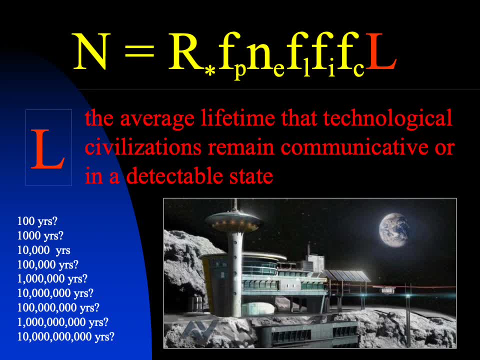 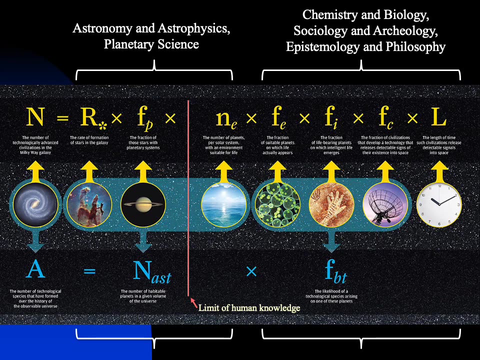 existence by the average lifetime L, and you get N, the number of technological civilizations that we could communicate with in the galaxy. Now, before we embark on each term and give each term a discussion, I just wanted to break them down a little bit about the type of science that's involved in each of these terms. 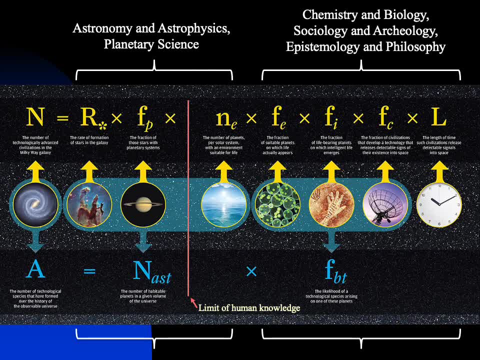 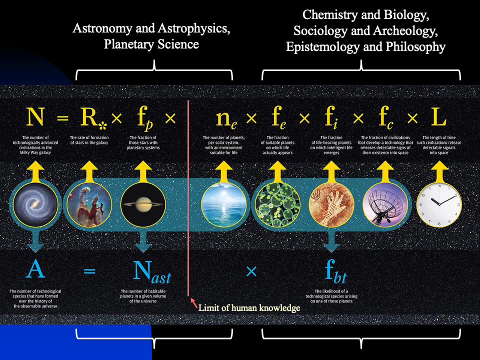 Now this is a handy-dandy little diagram that was put up by the SETI Institute, And you can see Drake's equation written in its mathematical form across the top: N equals r. star times f sub p times n sub e times f sub l times f. sub i times f sub c times L. 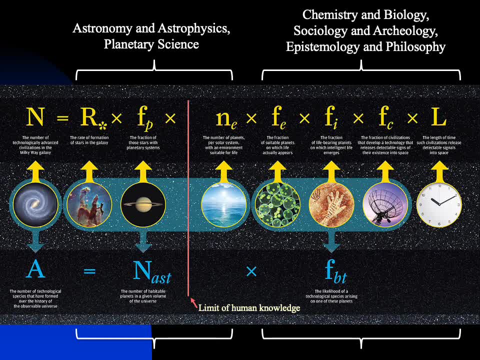 Let's talk about where the astronomy is. The astronomy is in r star, f sub p and n sub e r star- the rate of new stars forming in the galaxy every year. so that's clearly astronomy And that number has been measured pretty well. 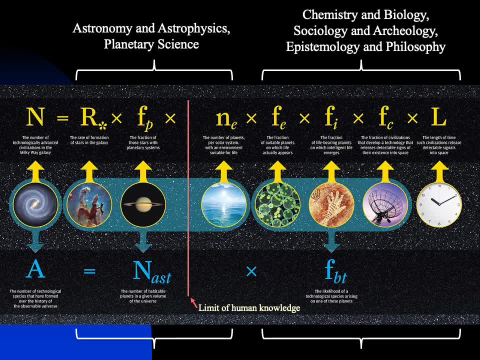 Then the fraction of planets, that, I'm sorry, the fraction of those new stellar systems which, for instance, form planets with them. that's also clearly astronomy. Now I've drawn a red line here, because that is basically the limit of human knowledge. 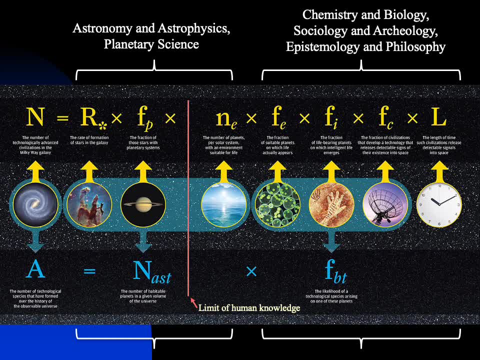 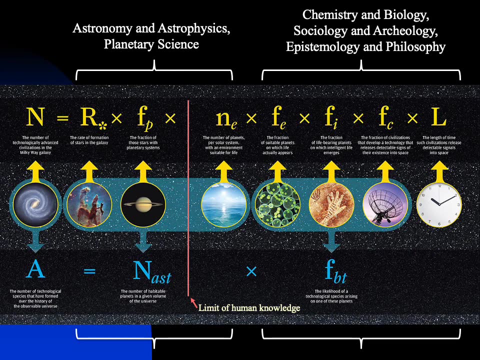 We have only in the last 10 years measured f sub p. We are now embarking on the process of trying to measure n sub e, And that we'll talk about later is also very much astronomy. So you can see, there's this, these pictures of 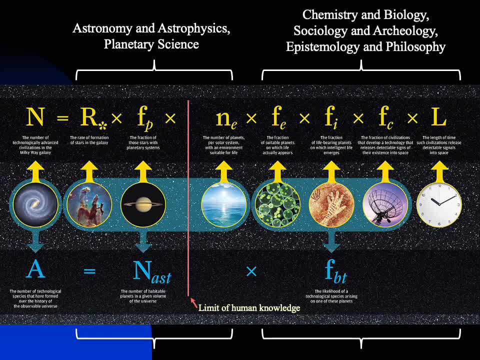 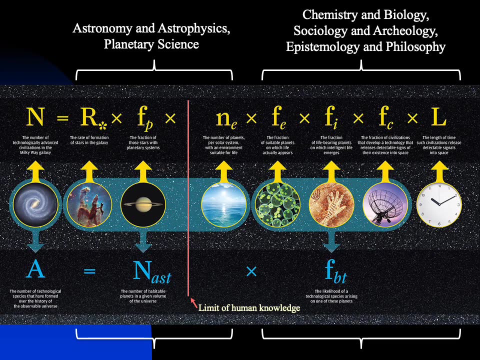 underneath the equation, these little diagrams showing the pictures, and there's this blue bubble and it has a little arrow down to it, n sub a s t. So that's basically talking about a s? t, meaning astronomical sciences, And you can see that I've drawn the red line bisecting that bubble. 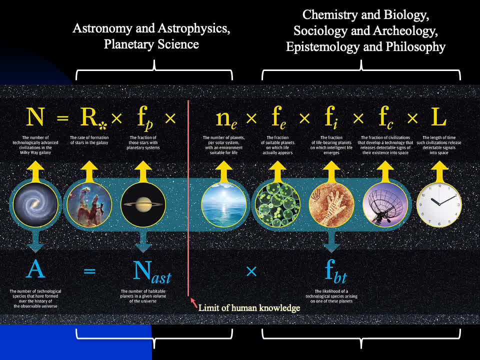 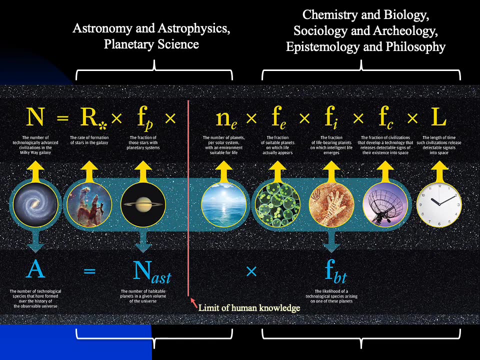 such that n sub e is on the right-hand side and represents areas where we don't have. we have not measured that number yet. So we are about two thirds the way through the astronomical terms that go into the Drake equation. Now, once we move on beyond that, we sort of get into the biological aspect. 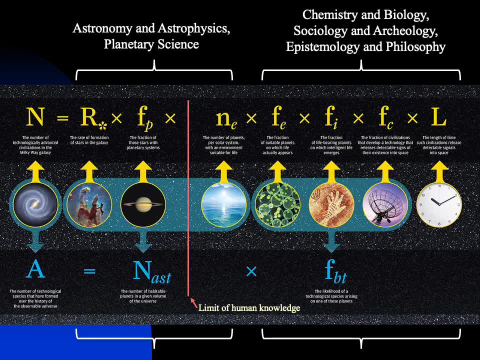 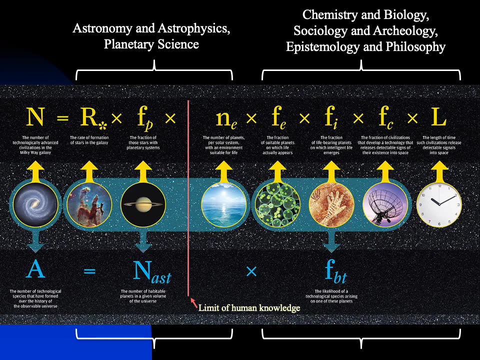 and technological aspect or intelligence aspect. So the chemistry, the biology, the sociology, the study of knowledge itself, epistemology and the philosophy that these beings will have about who they are, what they are, how they want to exist and why they exist, all is couched in the terms F sub L, F sub I. 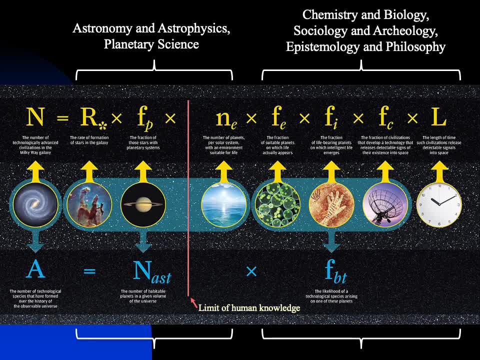 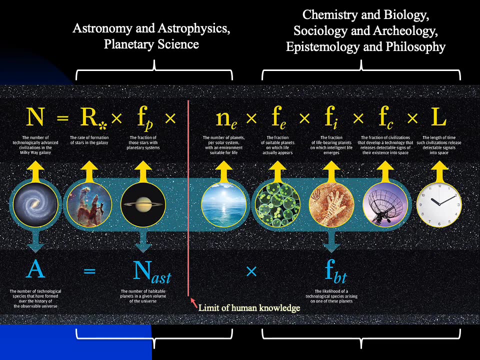 and F sub C, And you can see that there's a blue bubble around those terms as well, And so the product of these give you basically the fraction or likelihood that life forms and becomes intelligent and develops technological civilizations. We basically have sparse data on 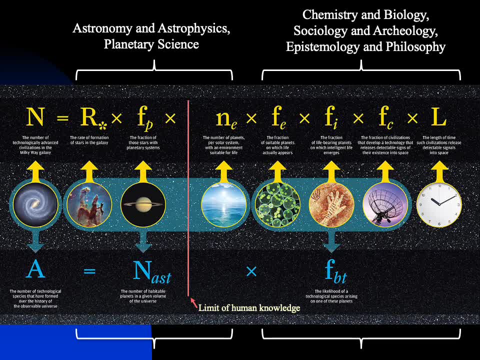 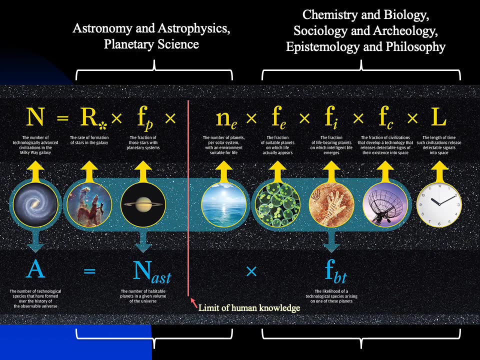 the planet Earth to help us with that. But other than that, we have no astronomical context by which to estimate these numbers. And of course, last on its own is the average lifetime of the civilization L, And that again is going to come down to societal behavior and philosophical 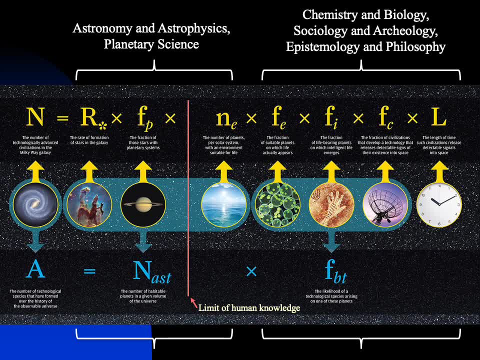 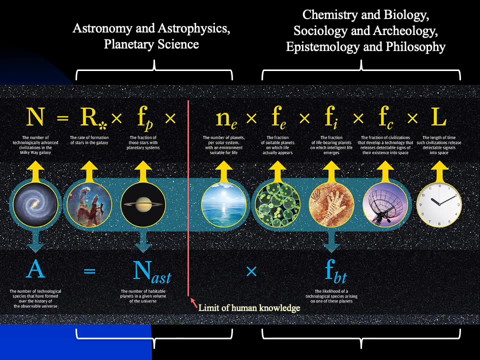 understanding self-understanding of the beings as to whether they have a strong urge for self-preservation Or whether they, in the end, are not highly enough intelligent to preserve their species and their technological civilization. So I just wanted to review this with you one more time. 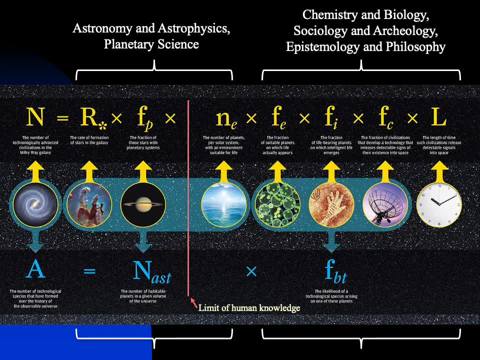 that it's broken up into these areas of human knowledge, that we have done probably good measurements of two of the terms. astronomically, We're, in the next 10 years going to probably nail down N sub E and then have nailed down the astronomical data. So I just wanted to review this. to give you a general understanding of this. Maybe you can see something about undeniable evolution in the alcohol community at the end of today's session. So what it's called is the graph and it looks like this graph, but don't worry about the mathematical terms. 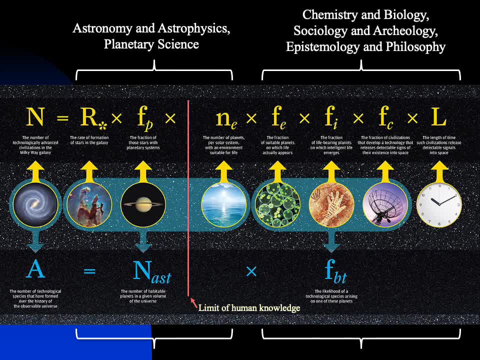 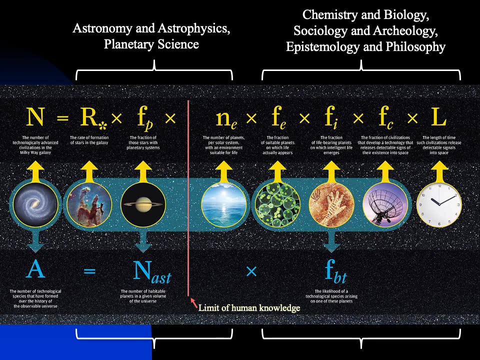 And then it's up to the biologists, neurobiologists, and hopefully, if we find life in our own solar system, we can learn something more about F sub l other than information that is on Earth. So now we're going to go through each of the terms in the Drake equation, For those that we've 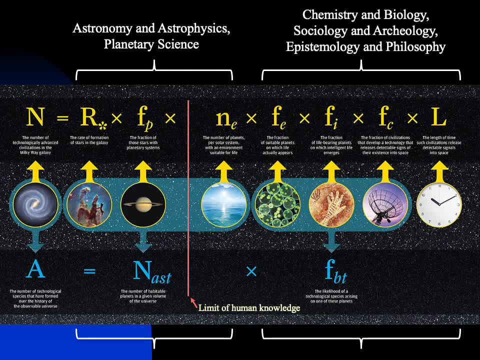 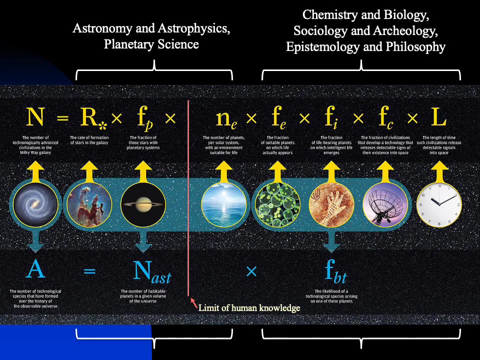 discussed earlier in the class in terms of previous chapters that were modeling this, the we've discussed. I'll spend less time on those and what I'd want to do is spend more time talking about basically, f sub i and f sub c and L at the very end. 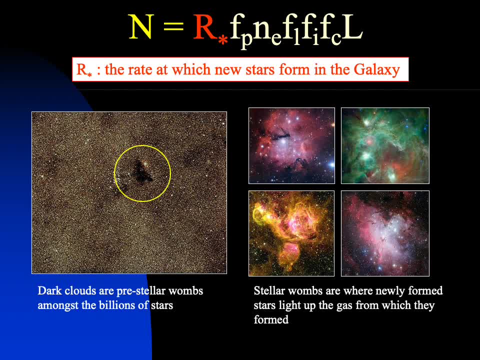 Okay, so let's start with r star. I remind you again that the letter that we're talking about, or the variable we're talking about, is always in red, and I put the definition of that term in the white box up top there. So 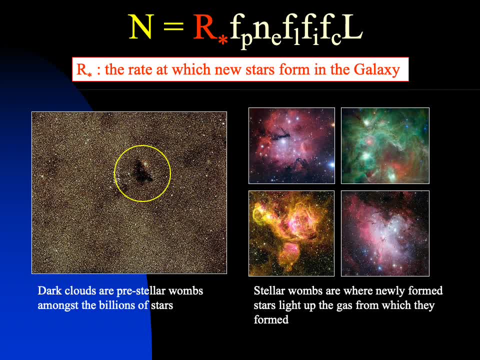 basically, r star is very well measured. We've had good measurements of r star, say, from the 50s and 60s onward in the galaxy and we get better at it all the time, but it's a well-measured number. And just to review quickly the 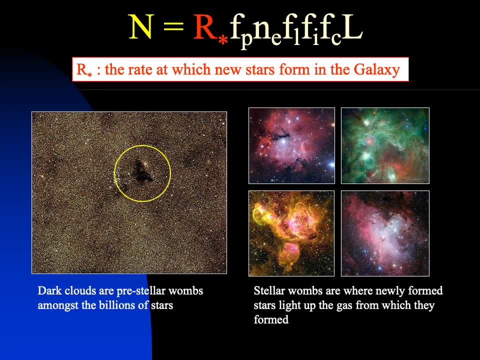 pre-stellar wombs are basically these dark cold gas clouds such as the one you see here, Circled in the yellow on the left diagram, And then, after the stars form, they light up and you see these stellar wombs, And so I showed some various 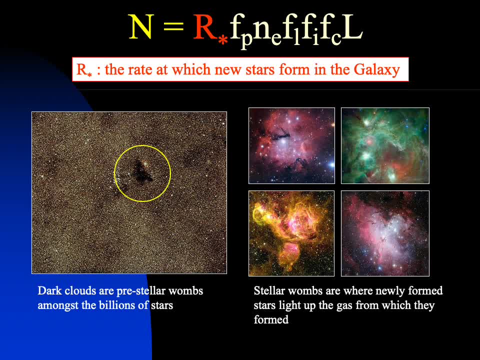 pictures of these stellar wombs for you. And these stars light up, and then they blow the gas away, and many of these stars, of course, form planets around them. Now, these stellar wombs are not just located willy-nilly and random in a 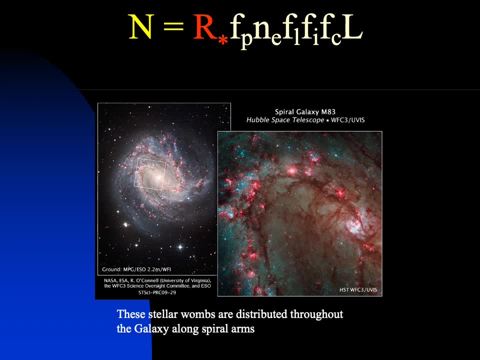 galaxy. So here's a picture of a particular galaxy And in this galaxy you can see that there are these stellar wombs and they seem to be lined up along these stellar. I guess we should call them spiral arms in say this galaxy. that's like rotating. If you expand the picture on the left. 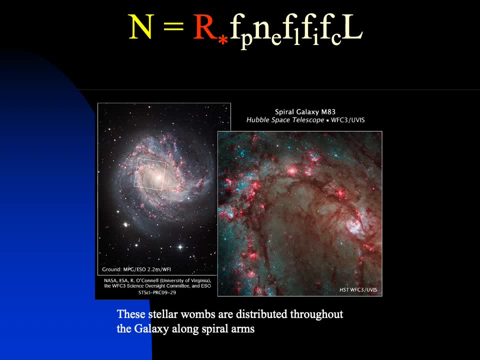 equal to that little box that you see in there and look at it in detail. you can see the dust lanes Right where the dark clouds are. those are the pre-stellar wombs. You can see the lit up red clouds. those are the stellar wombs where stars are forming And then of 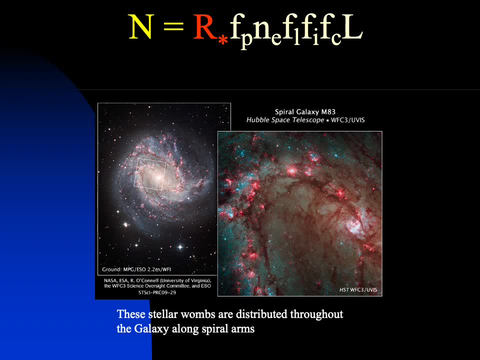 course, near them or around them, you can see where the stars are emerging from. the cocoons are sort of the blue areas And you can see this is all highly structured. This is going on and it's a large ecosystem, a big physical process. 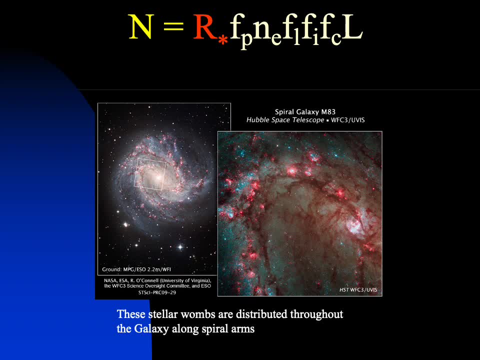 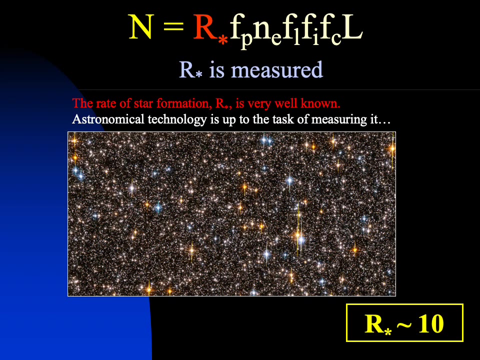 We reviewed this in one of our previous lectures, but the point I wanted to say was that the galaxy is an ecosystem, and this is happening at a regular rate all throughout the galaxy and in a very organized way. So from all of that process that I just discussed, you get a lot of stars And, in fact, 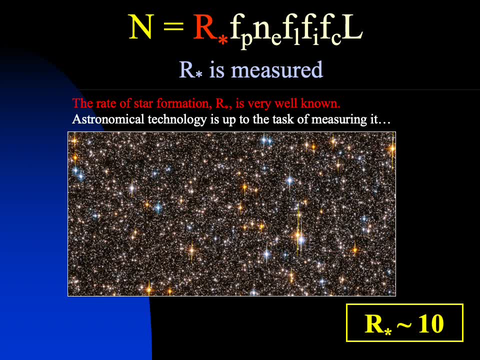 currently, the galaxy has somewhere between 200 to 400 billion stars in it, But what we're going to do is we're going to take a look at the galaxy and we're going to take a look at the stars And what I'm emphasizing- the process of how the 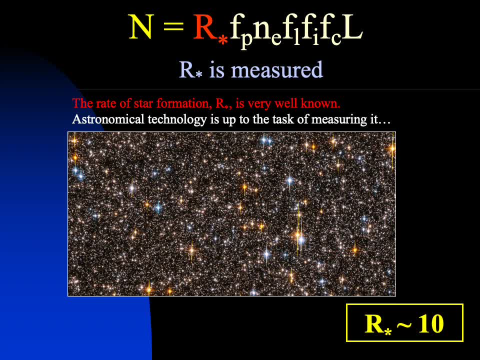 stars are born and how they form and the rate at which they form. When we look at all these clouds on our own galaxy and we measure the rate at which new stars are forming every year, it turns out that we get a number that's around 10.. So 4. 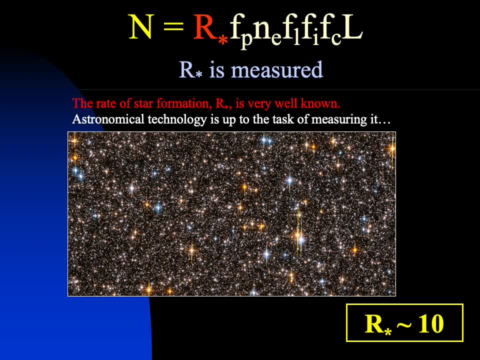 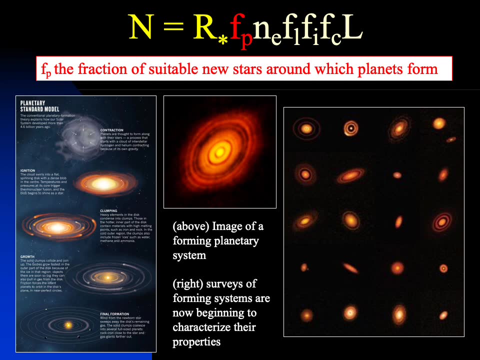 are the Milky Way galaxy. our stars measured quite well and that number is on the order of about 10 new stars that form in the galaxy every year. Now we move on to the second term of f sub P, the fraction of suitable new stars. 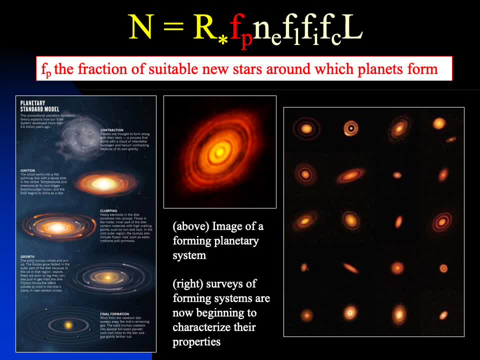 around which planets form And, as I was explaining, this is something that we have made very good progress on over the last, I guess I should say, 15 years. The first exoplanet planted around another star was discovered in 1995.. Since then, we've had a relatively wideщё�rocent of exoplanets around another star. 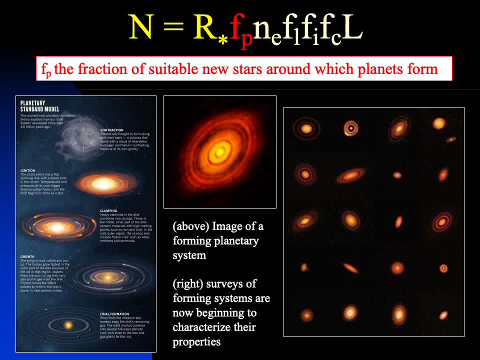 appliedツ 65 quatro in 1995. Since then we've had Hosts- more than 220 accounts", a lot of space missions and ground-based missions that have tried to attack this problem. One of the things that we learned was that our standard model of 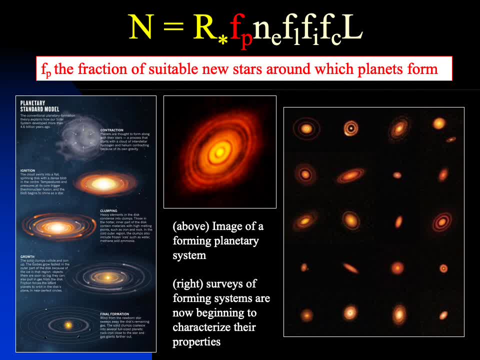 planetary formation was significantly challenged. You know, we talked about the method of which science happens and we had our solar system to study and we put together some hypotheses on how our solar system formed, And so there are several steps to that and I'm just illustrating that in the diagram on the 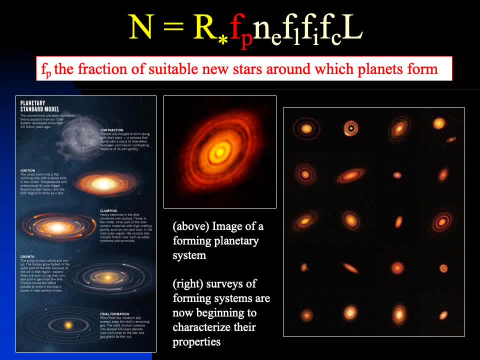 left. It's not necessarily that we have to review that process again, but it's a process of gas contraction followed by coalescing of planetary sized bodies, And the idea was that rocky planets would form toward the inner parts of it and gas giants would form toward the outer side of it. And we have new. 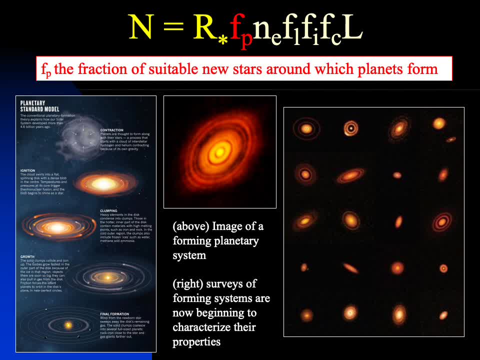 information on the solar system. that would suggest that our planetary system did not form so simply as that, and because of the distribution of planets that we found around other stars, which I'll talk about in a minute, it's pretty clear that not all our solar 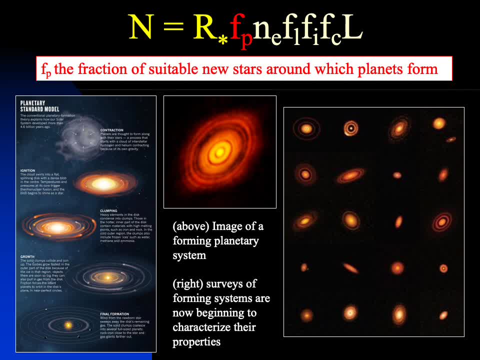 systems, not all other stellar planetary systems, I should say, look like our solar system Now in the middle. I want to show you an image that's taken from the ground, in the submillimeter and with a ground-based telescope that's called ALMA, from South America And, as you can see, 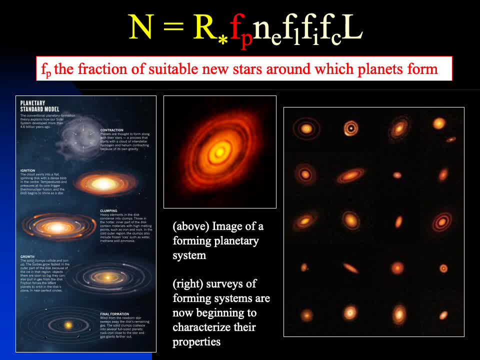 it is able to resolve the formation of a planetary disk And this is very interesting and you can see some clearing out where there's dark rings and these are believed to be areas that are cleared out by the presence of forming planets or forming large bodies And the emission 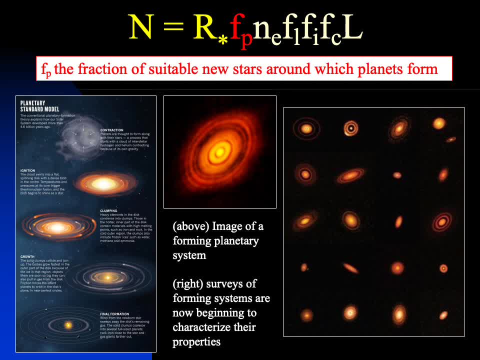 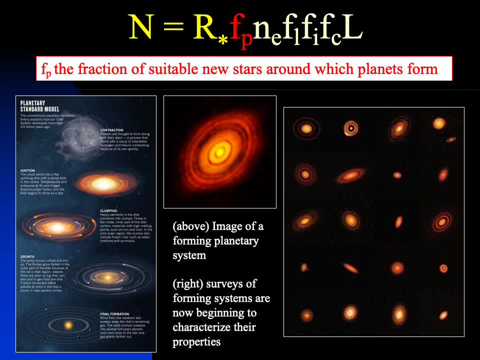 of it in the infrared as well. That's a diagram of one such system. On the right, I'm showing you sort of a postage stamp of various systems that are in the process of formation. So we have a great deal of new knowledge about the various time steps that are going on. We can look at the 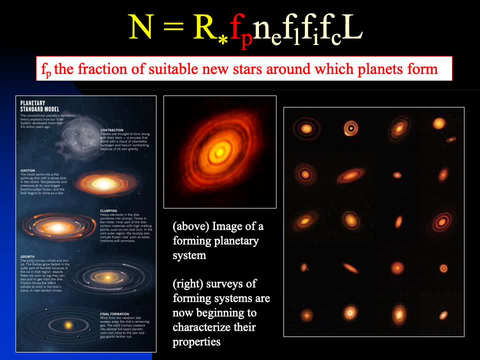 evolution of the formation of these planetary disks and planetary systems and look at the distribution of the kind of planets that come out of it. So this is a very, very interesting thing, that tool that helps us understand empirically meaning with data, not just looking at our 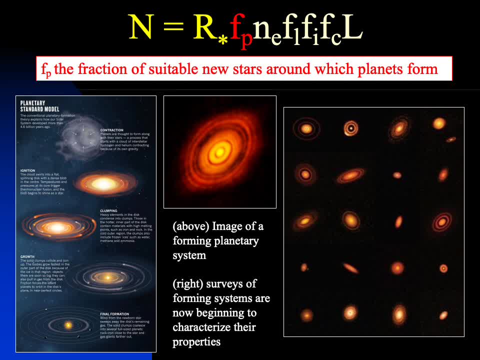 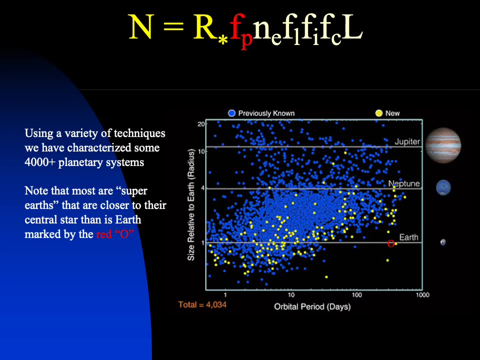 already formed solar system and making guesses or applying physics and hypotheses, but actually looking at the distribution of the various planetary systems. Okay, so what is the distribution of planets? look like around other stars, And so this is one diagram of many that you can find on the internet that shows you the distribution of planets. 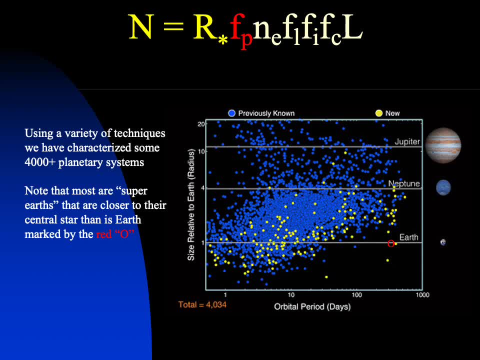 Now plotted on. this particular diagram is along the x-axis is the orbital period in days. Now Earth has an orbital period of 326 days, give or take some fractions, And so it is toward the right-hand side between the 100 and the 1000. there, Just so you understand how the graph is read. 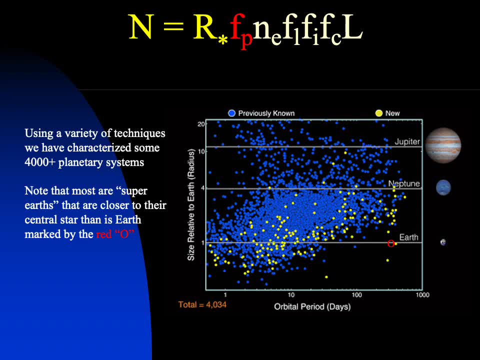 it's a log graph And so you can see where the one is. And then the next tick is two, three, four, five until you get to 10.. And then, as you go from the ticks to the right of that, it goes 20,. 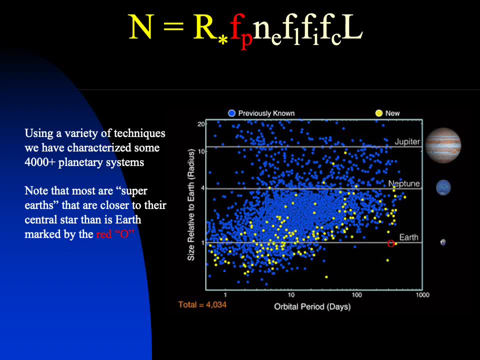 30, 40.. 50, 60, up to 100. And then in that decade it goes from 100, 200, 300, 400, up to 1000.. So this is a log plot And you can see that where 300 is on that graph. Now the vertical axis: 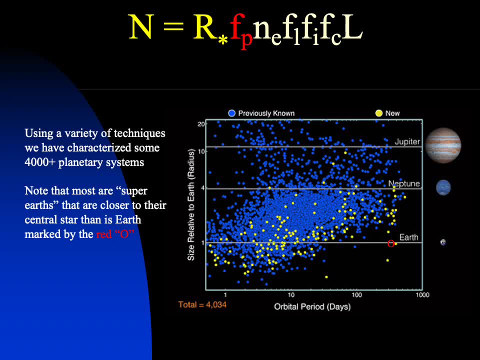 the y-axis is the relative size of the planet compared to the Earth's radius. So the Earth's radius on this is one. And this is a little bit of a log plot, in the sense that it goes from a number below one up to 100. And then it goes from a number below one up to 100. And then it goes from a number. 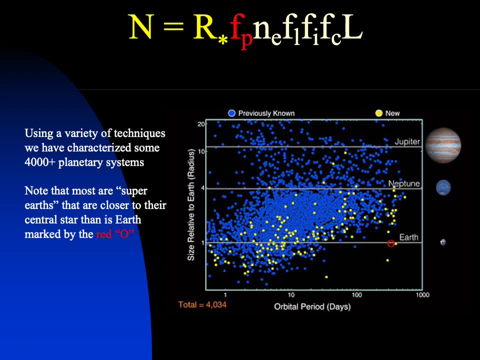 below one, up to about 20.. And so the first line, the lower line, is the Earth's radius, And so you can see now I've put this red circle where the Earth would reside on this diagram, And it has obviously one Earth radii, and it's out at 300 orbital period days. And then of course, there's 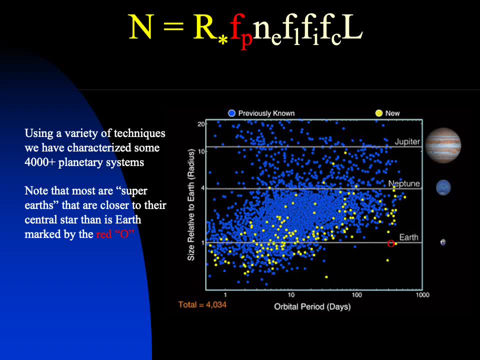 a nice little diagram of what the size of the Earth looks like, to the right of that line, And as you move upward we're going to see a little bit of the Earth's radius, And then, of course, there's a little bit of the Earth's radius, And then, of course, there's a little bit of the Earth's radius, And then 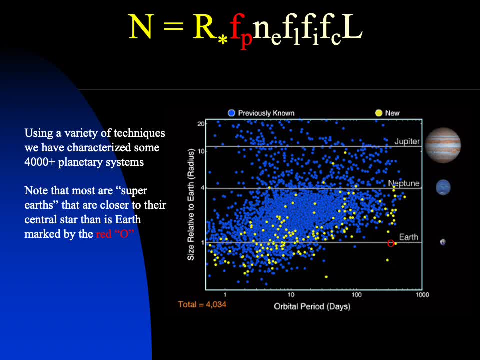 esempio, you get up to about four times the radius of the Earth, You're looking at Neptune-sized planets. And when you get up to a little over ten times, maybe eleven times, you're at Jupiter-sized planets. okay, A lot of planets are being formed. So every time they make this diagram- because 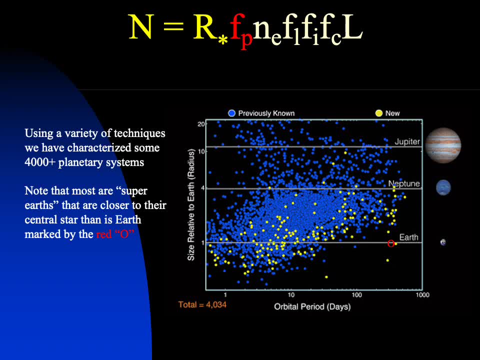 we're discovering new ones all the time. they always show the new ones versus the ones that were previously known, But what I want you to do is look at the distribution and you can see that there And remember that this is always a gigantic memory, while for themnot everybody can actually save it. If 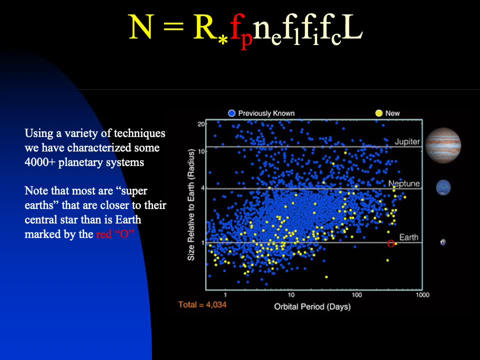 are a lot of planets that have the radius of the Earth, But if you look at the most common type of planet, it's really what we call a super-Earth, And a super-Earth is a few times the mass or the radius of the Earth, I should say, And there are much fewer Neptunes and Jupiters, So that's pretty. 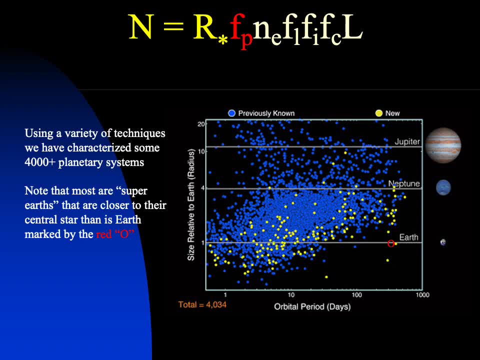 interesting that most of the planets that form in our galaxy around other stars tend to have sizes that are a few times, somewhere between the Earth's size and four times the size of the Earth. Now, the orbital period is a little bit tricky of a number. It doesn't exactly give you distance out. 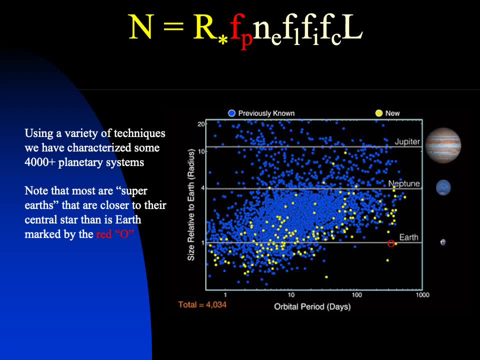 okay, because it does depend a little bit on the mass of the star. Not all stars have the same mass, So you have to include the fact that the smaller mass stars, the planets that might be in their habitable zones, might have the same mass. So you have to include the fact that the smaller mass stars. 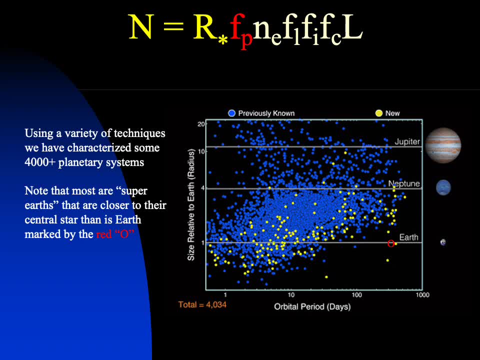 have shorter period days, And so it could be that some of these planets that have orbital periods of about 10, and you can see there's a lot of them- super-Earths that have those kinds of orbital periods. they might be around much lower mass stars. So it's hard to imagine living on a planet. 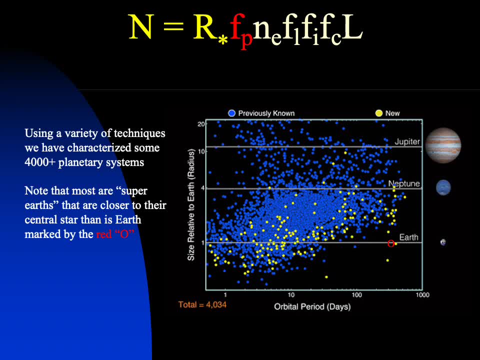 in which the year is only 10 days long, but that tends to be more typical than a year that is 300 and something days long. So the point is in the bag. we have found and measured some of the properties of some 4,000 planetary. 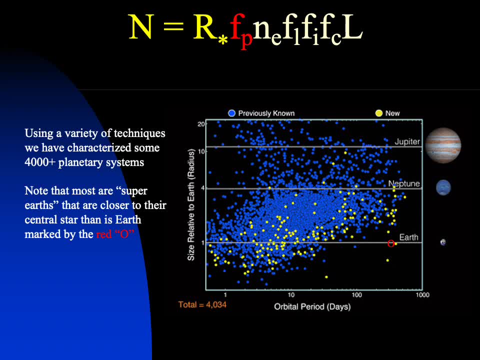 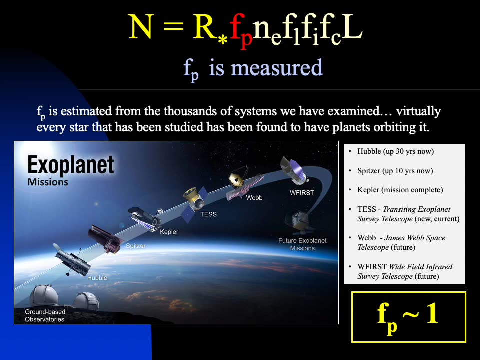 systems, And this is showing a distribution of those sizes and distances from, in a sense, distances from the central star. So, in the end, is F sub p very well measured or is it not very well measured? And the answer is that it's pretty well measured. Now, why do I say that? Because this is a fraction. 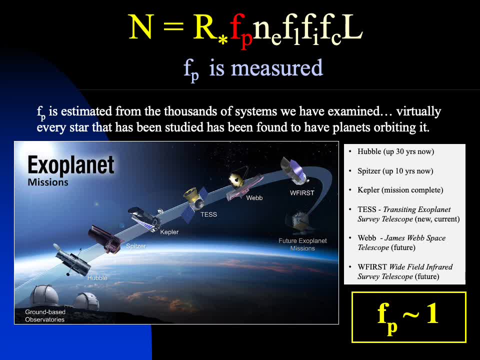 out of all the planetary systems that do exist, or I should say out of all the new stars that are coming into existence, what fraction will have planets around them? And what we found is that, no matter what star we look at, we tend to find planets around it. It's not exactly 100%. In other words, 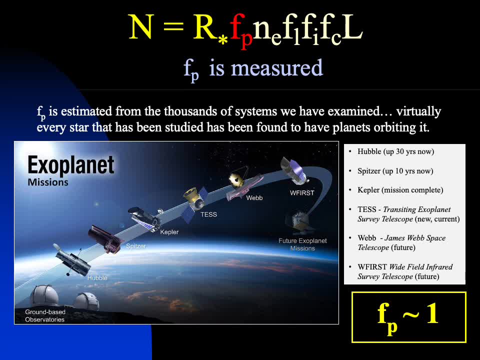 F sub l is not exactly one but it is. Everything goes pretty darn close that pretty much you can approximate F sub l as, I'm sorry, F sub p as being one. Now I want to talk very briefly about the future and where we've been with this In this diagram before here. 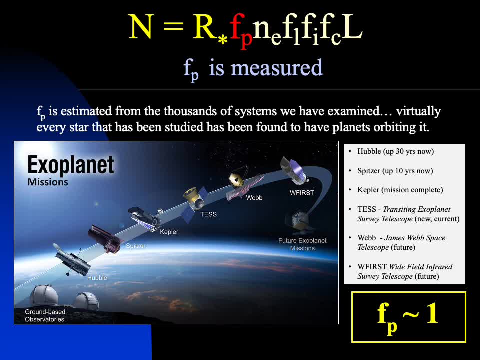 you can see, ground based observatories have played a role And in 1995 was the first time that a ground-based observatory detected a planet around another star. We've had Hubble since 1993 and spitzer since the 1990s. 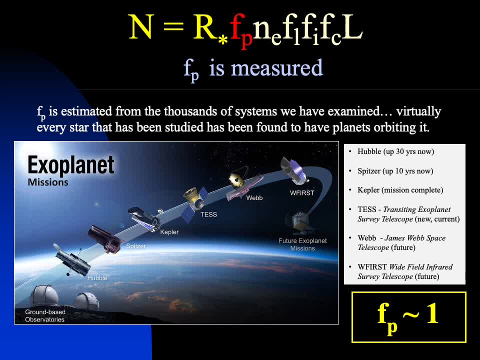 and then, in the 2000s, we launched Kepler. Kepler is a mission that well. first of all, I want to say that Hubble has been going on for 30 years and is still up, and Spitzer is also still up, even though it's not doing its primary mission anymore. Kepler is a mission that came and went, but 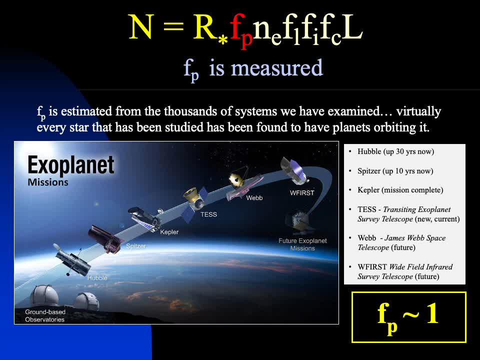 discovered many, many of these planets. So the new satellite that's up is called TESS, the Transiting Exoplanet Survey Telescope, and this is meant to find a lot of Earth-like planets around, or super-Earths around, other stars, And coming in the near future is the James Webb. 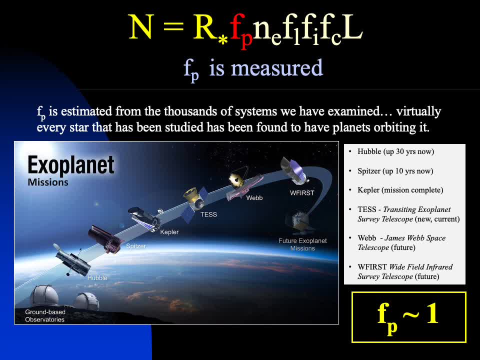 Space Telescope and this telescope and the next follow-on telescope which should come in the next decade, WFIRST Wide Field Infrared Survey Telescope. those are both designed to find more information about the next term in sub-E, In other words, measuring properties of the atmosphere, trying to determine which ones have. 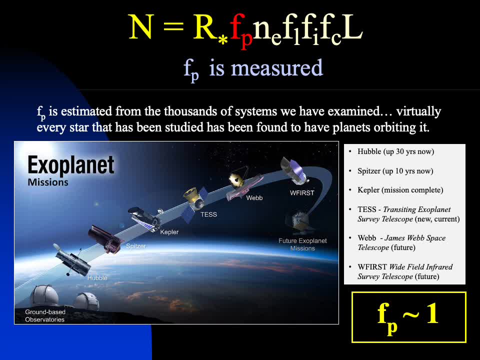 are habitable planets and which ones are not. So those future telescopes coupled with TESS to find many, many, many, many more of these candidates, would follow up with Webb and WFIRST to actually determine which ones are going to have habitable atmospheres. or 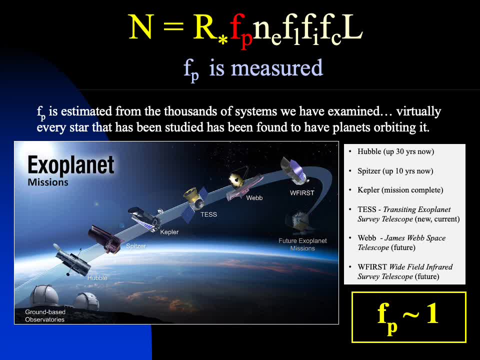 surfaces. So in the end, coming back to Fp, it is well measured and is on the order of one. And now we're going to move to N sub E, but I wanted to show you some of the telescopes that are going to help us understand and measure N sub E. Now we move on to the next term, N sub E. I want to remind 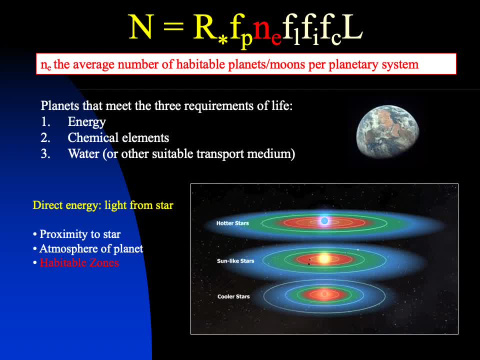 you that N sub E is a number and it's an average number of habitable planets or moons per planet system. Okay, and what we mean by habitable is that planet has the three requirements of life: energy, chemical elements and water or a suitable transport medium. Now we had some good arguments. 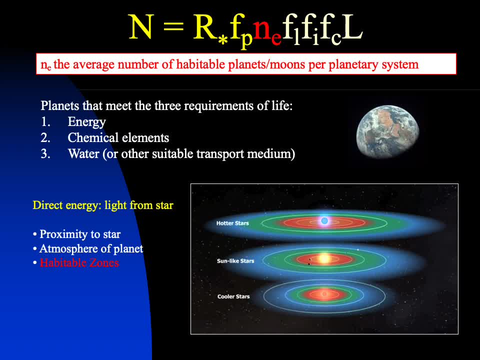 in previous lectures in the course, as to why water is hands down the winner when it comes down to being a suitable transport medium for metabolism. Now we also discussed the inverse square law of light, that the light from the star decreases with the square of the distance from the star. 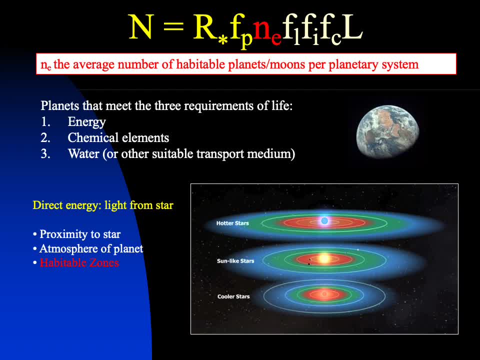 So proximity to star relates to the energy. So this is very important. You know we are talking about planets, We're talking about where they are relative to a star, and so the amount of energy they receive from the star, the total energy budget, if you will, of many planets, is dictated. 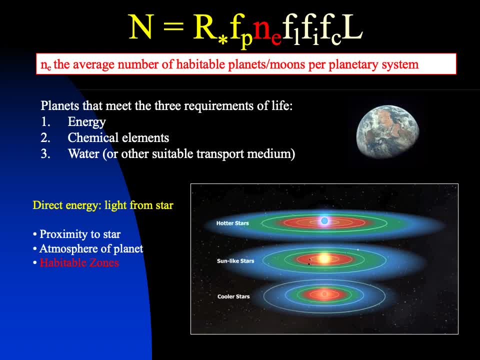 by how far away they are from the central star. We also discussed the habitability in terms of the atmosphere of the planet and what its chemical composition was, that some of them were stable for liquid water and some of them were not, and that those two things came together in a concept called the habitable zone. 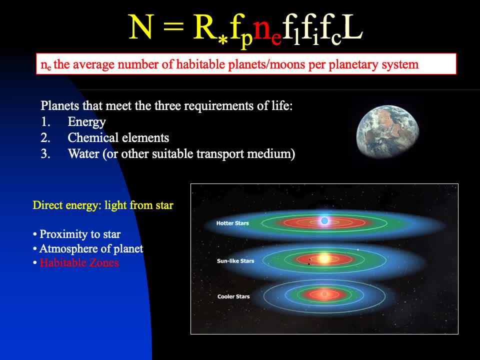 So I just want to show you, with this diagram in the lower right, that the habitable zone does depend upon the luminosity of the star. Okay, we did discuss the habitability of the star, the evolution of the sun, and that the sun is getting more luminous as it ages and therefore, 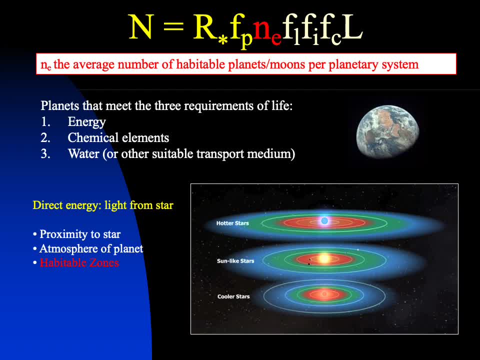 the habitable zone of the solar system is moving outward, okay, with time. So in these diagrams, where green is showing you the Goldilocks area, the habitable zone, blue is showing you areas which have too low of energy, too cold in a sense, and orange showing you areas that have 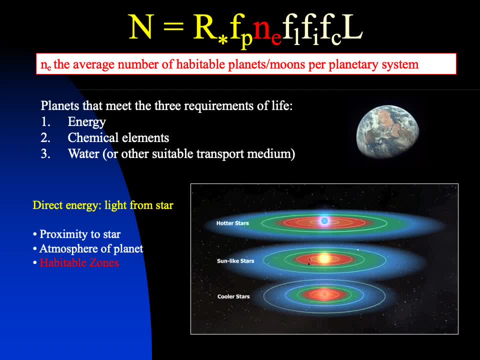 too much of the sun's or star's energy are showing and the orange And, as you can see, when you go from cooler stars, the shell of life, the green habitable zone, is actually much more narrow and smaller in radius, And as you go to hotter stars, 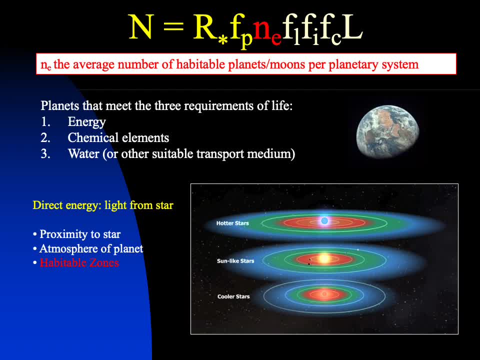 you get much larger habitable zones that are further away And I believe in each of these diagrams they're showing the orbits of the inner Mercury and then Venus, Earth and Mars And you can see that for the sun-like star you have, Earth is well inside the habitable zone, Mars in the outer edge. 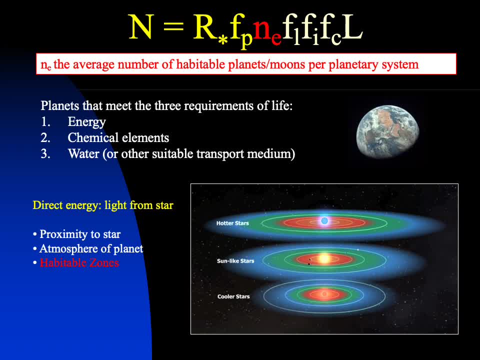 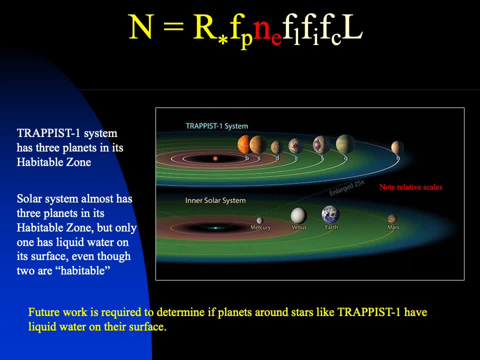 and Venus inside the inner edge. Now discussing habitable zones, just a little bit more. we might want to know something about what the habitable zones around all of these other stars in the galaxy are like, And of course, they depend upon the star's luminosity And it turns out the luminosity depends upon the star's luminosity. 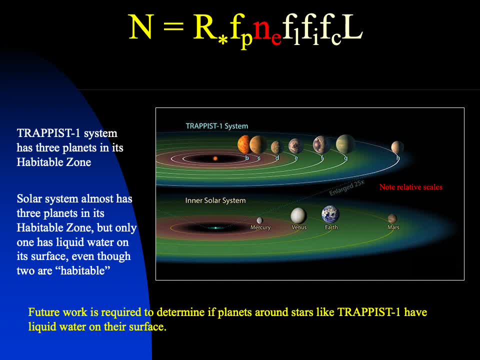 And it turns out the luminosity depends upon the star's luminosity. And it turns out the luminosity depends upon the mass of the central star. We'll be talking about more about that in our next module, But I'm introducing the idea to you right now. So in the bottom of this diagram we have the. 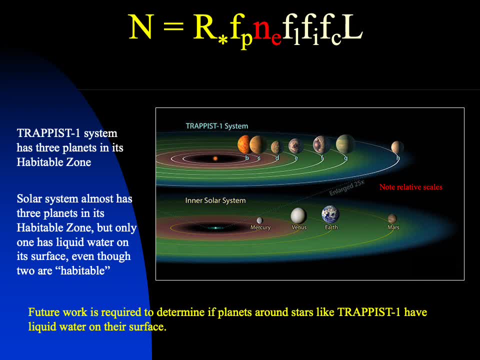 inner solar system showing Mercury, Venus, Earth and Mars and the green habitable zone, And this picture tends to show Venus just being on the inside of the habitable zone and Mars just being on the very outside of it, But in fact our estimates would show that the 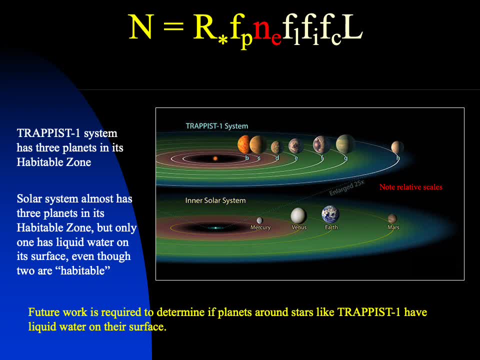 habitable zone is a little bit smaller than the inner solar system, And so we're going to have to be a little bit narrower than that, and that Mars and Venus are really currently not in the habitable zone. So this diagram is not 100% accurate, but pretty close. Now I'd like you to show you the 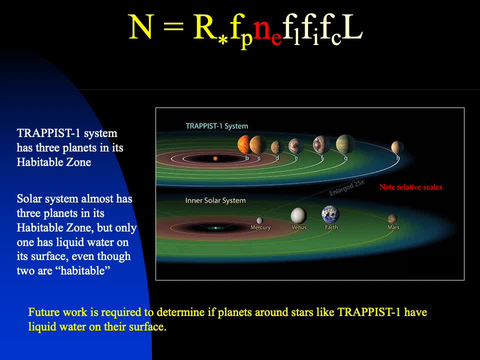 habitable zone around the TRAPPIST-1 system. This is just one of 4,000 systems for which we have measured multiple planets orbiting around it. Now I want you to understand. the scale of that system is very, very much smaller than our solar system And in fact, the scale of that system is very, very. 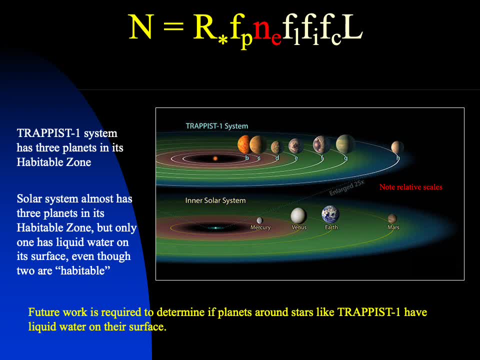 small. In fact, you can see that these little dim lines are showing you the little inner region of our inner solar system, the very inner region near our star. in the bottom diagram. That is showing you the size of the upper diagram. Okay, and so basically all those planets would fit. 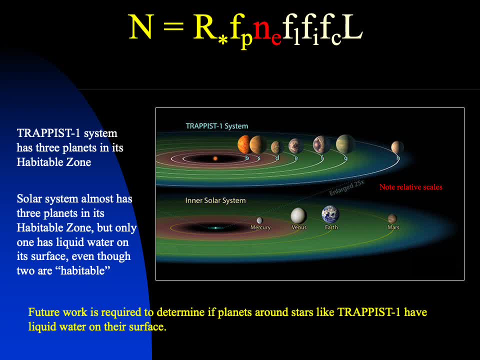 well, well, inside of Mercury's orbit around the Sun, The TRAPPIST-1 is a very low mass, very low luminous Star, and so its habitable zone is in close. But what's fascinating is three of its planets. 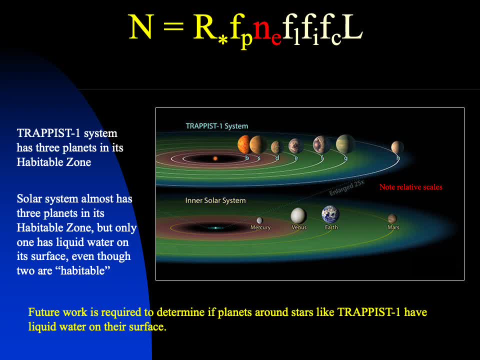 E, F and G are actually located in TRAPPIST-1's habitable zone. So here's a situation where, with the solar system, one planet is currently in the habitable zone, But at one point in time you might have said three were, depending upon Venus and Mars, and all of that. 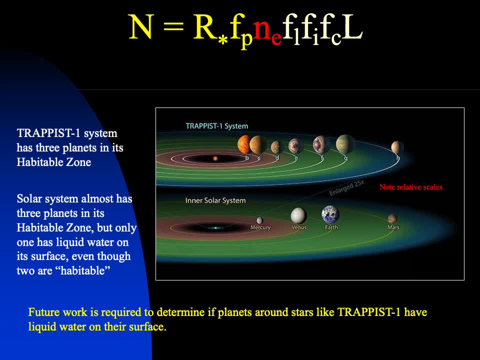 But in the TRAPPIST-1, we definitely have three that are currently in that habitable zone. Of course they change with time, But you know, we want to know is the average number of these planets that are habitable Now? just because a planet's in the habitable zone does not mean that. 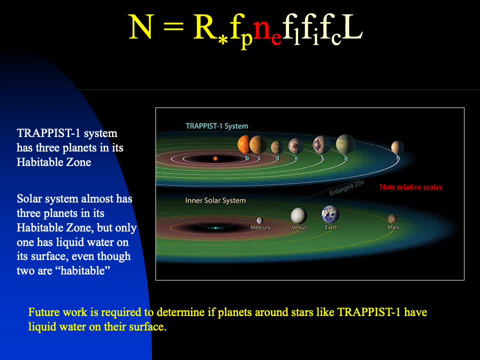 it is habitable. Okay, so just knowing the number of planets in habitable zones doesn't give you N sub E, or averaging those numbers doesn't give you N sub E. We also want to account for other possible situations where a planet or moon could be. 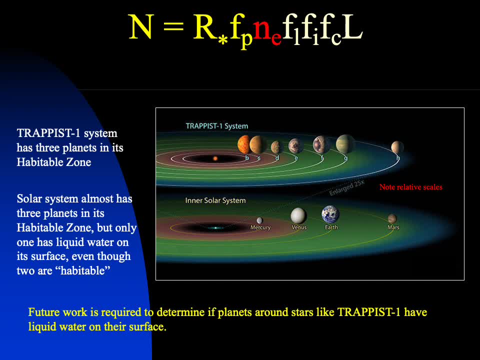 habitable, which we'd have to add to our term if we were able to count the number of habitable planets in habitable zones. So future work is going to be required to understand which of these planets in TRAPPIST-1's system are indeed habitable, And that's where I told you about the 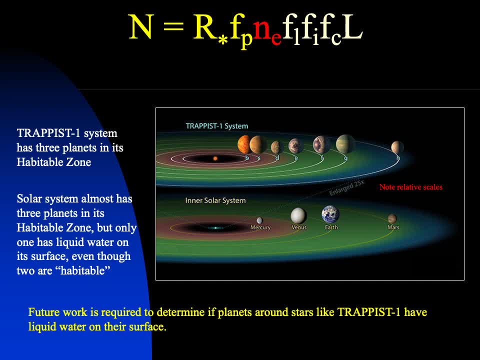 JWST and the WFIRST missions that are coming up. So that's where I told you about the JWST and the WFIRST missions that are coming up. They'll be doing work like that, Okay. so N sub E is definitely on the radar in the crosshairs for science. that is being done in the next 15,, 10, 15. 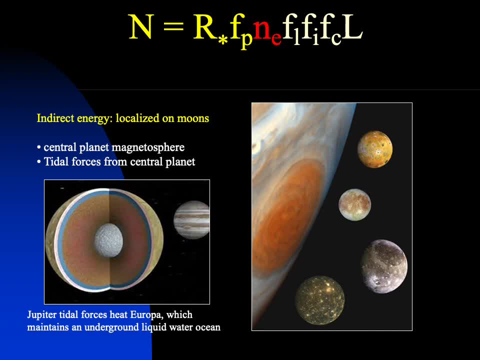 years. In addition to habitable zones and planets that are in habitable zones, as opposed to habitable planets that are in habitable zones, which is what we're really after as part of calculating N sub E, we also discussed in this class the type of planets that are in habitable. 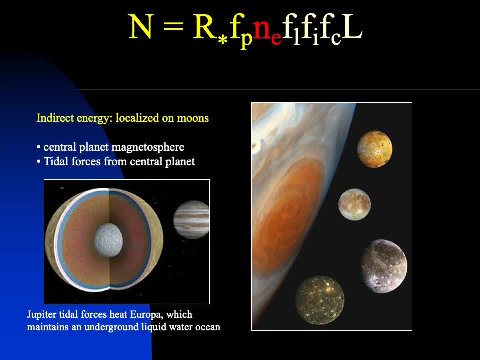 forces that were on the moons of Jupiter and how they were in resonant orbits and how that caused a situation where, for billions of years, they were continually and continuously being tidal heated, And so you had moons like Europa, where you have an underground ocean and you have 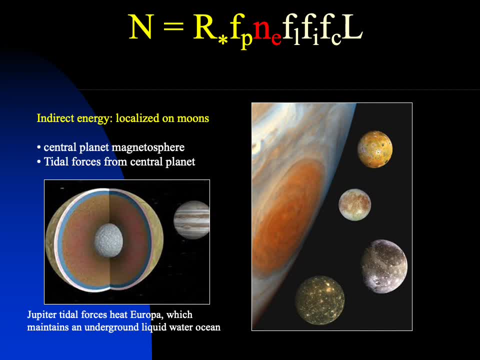 a surface ice layer around the top of it, There's definitely a habitable environment. It has transport medium, it has energy and it has the chemical element For life. Now it doesn't have quite the energy budget that Earth has, So if life was there, 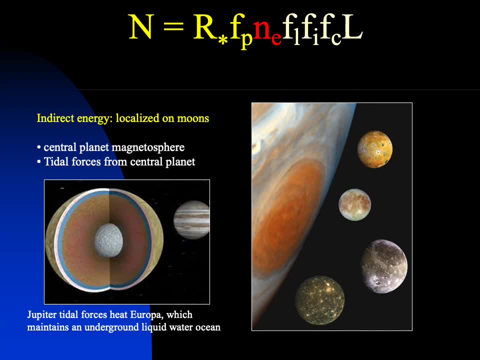 it may not be necessarily able to become intelligent life, But we're not there yet. in the equations You have to understand that We're not trying to pick out habitable planets at this point. for this, for calculating N sub E that we think intelligence will arise on, No, 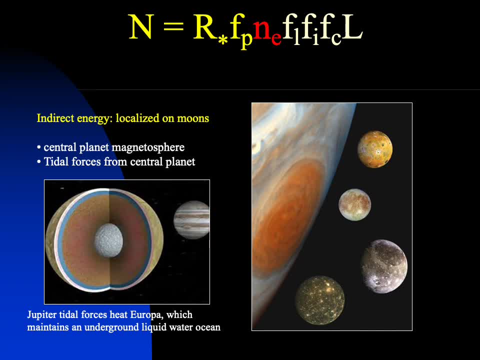 we are slowly, by slowly, applying our filters to this equation And, at this stage, N sub E is just how many of the planets per average in a system of planets is habitable. And so, if you want to figure out, well, how many is that in our solar system? Well, 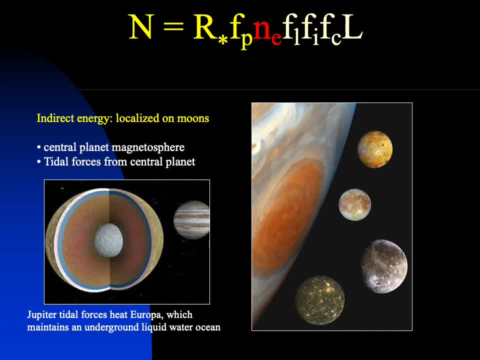 we could argue Earth is, We have argued that Mars is, And we have argued that Europa is. So we might use three for our solar system, Maybe in the cephalus, um uh, around um the planet, um. 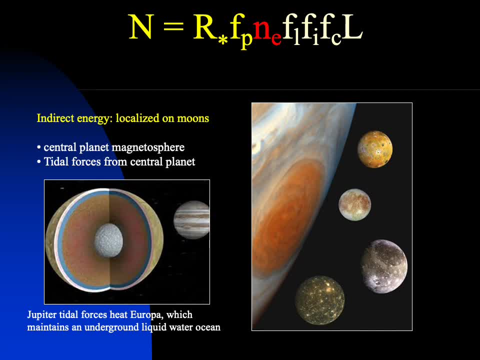 Enceladus? Sorry, Maybe Enceladus? uh, the planet around Saturn is also habitable, with its water geysers and whatnot. It has energy, chemical elements and has water and obviously a lot of energy. if it's sending geysers out into space and creating the E ring around Saturn, So maybe. 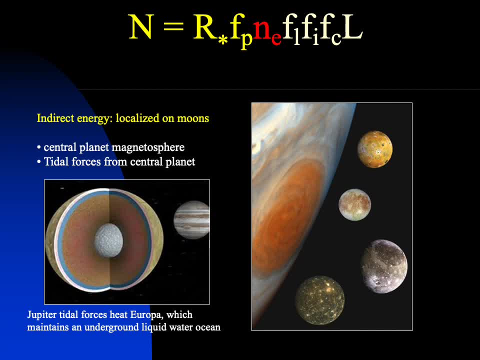 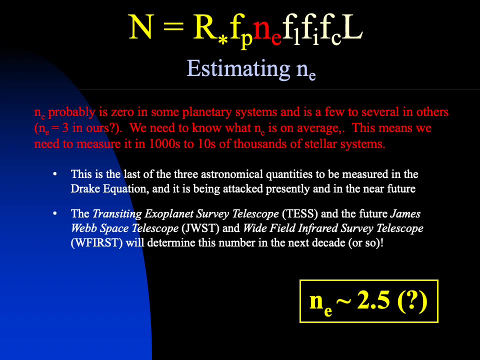 for our solar system. the number of habitable around um planets across all, instead of just available planets or moons- is around four. But the question is: what is it on average around all of these different systems that exist around, at all of the system that exist in the Galaxy? 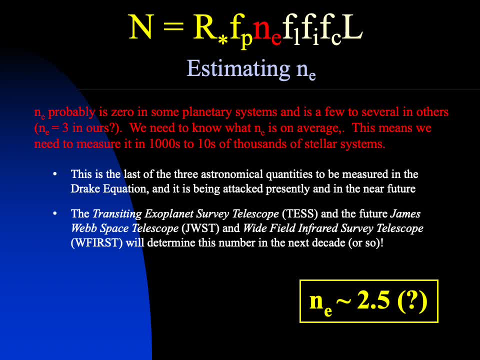 In the end, right now we can really not do anything but estimate in sub E, But we do know a few things about it. now We know something about how many planets are in habitable zones around other stars. uh, We don't know how many of them are actually habitable. 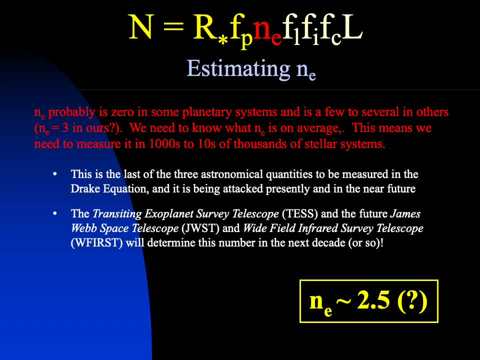 Ah, We don't know how many of them are actually habitable. That's currentlyThat's the question that's coming, as I've said before, and then we can use our own solar system as a guide. So in the end, as I've written in red here, it might be zero in some planetary systems and it 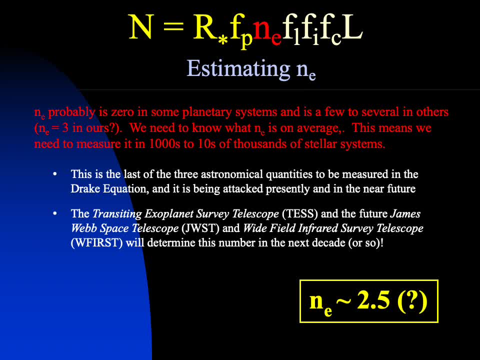 might be a few to several in others, and maybe in ours it's three, maybe four. We want to know what n sub e is on average across all these planetary systems that exist in our galaxy. So that would mean we need to measure this in thousands to tens of thousands of stellar systems in order to sort. 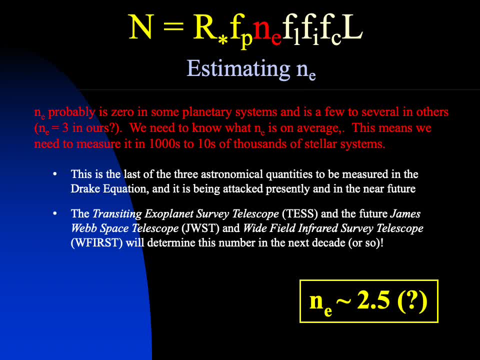 of get a nice average with small error bars on it. Okay, I want to remind you that this n sub e is the last of the three astronomical quantities to be measured in the Drake equation, and that is one we are presently attacking and will do so in the near future, reminding you that the Transiting 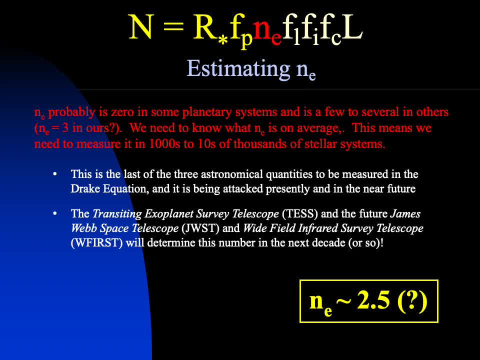 Exoplanet Survey Telescope and the James Webb Space Telescope and the Wide Field Infrared Survey Telescope will all be instrumental in doing that over the next 10 to 20 years. So you know, I think that we'll have some good answers within 10 years. 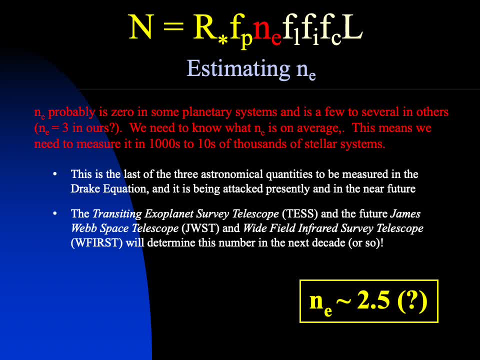 but certainly within 20 years we are going to have a very good estimate of n sub e and probably we'll have found, I would say, dozens of habitable planets in the galaxy. Now I have a question mark in my yellow box down at the bottom: n sub e. 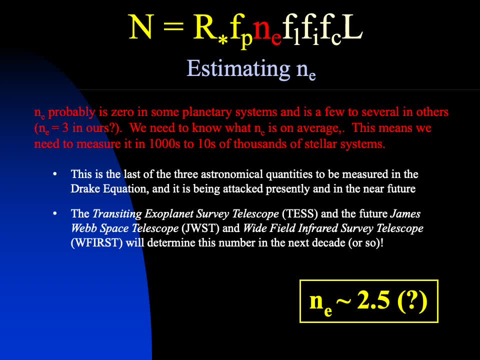 may be around two and a half. Okay, so how can you have two and a half habitable planets? Remember, it's an average. It's like saying the average family has 2.5 kids. Okay, so the average planetary system has 2.5 habitable planets. Of course we don't know the number, but that's just 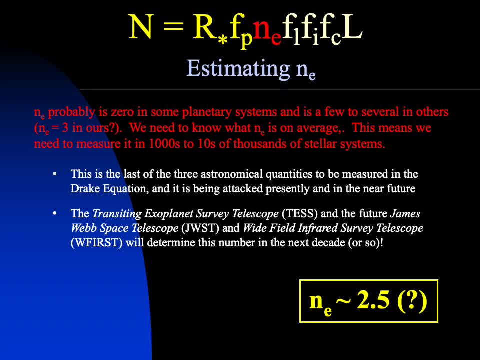 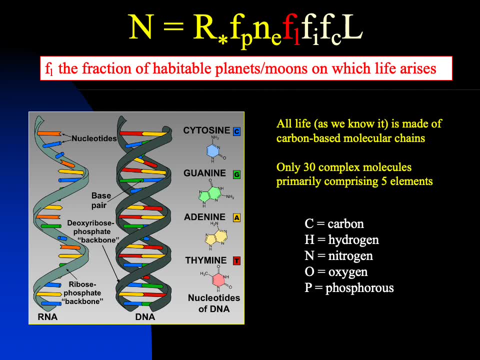 an estimate for now for us. So we're going to have to do a little bit of math here. So keep in the back of our mind Now, as we've taken our journey down, the terms of the Drake equation. you know, we've started with the rate at which new stars form in the galaxy, which is 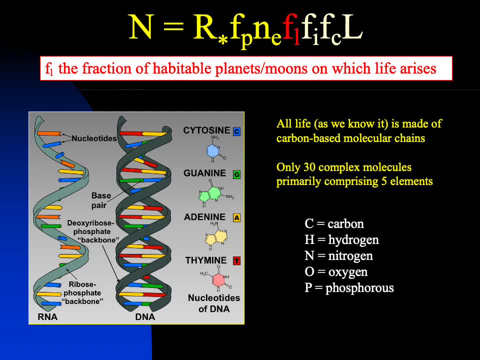 about 10 per new stars per year. We said that. then we multiply that by the fraction of those new stars which will have planets form around them. f sub p, which we said is about one. So that means we're getting about. 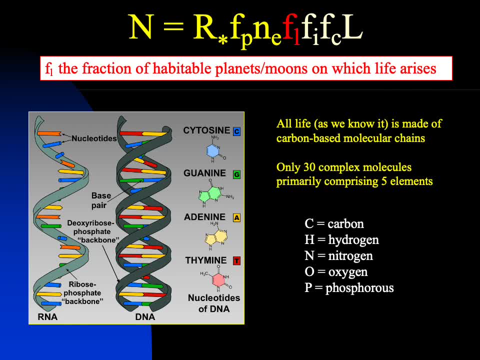 when we multiply those two together, we get 10 new planetary systems coming into the galaxy every year. And then we multiplied that by n sub e, the last of the astronomy terms, and that gives us the. when we multiply those three terms together, we get the rate at which new habitable 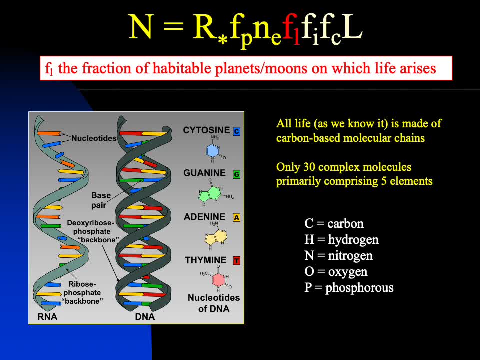 planets are coming into the galaxy And we said maybe that number's around two or two and a half or three. So we have 10 times one times two or three, And so we maybe have somewhere between 20 and 30 new. 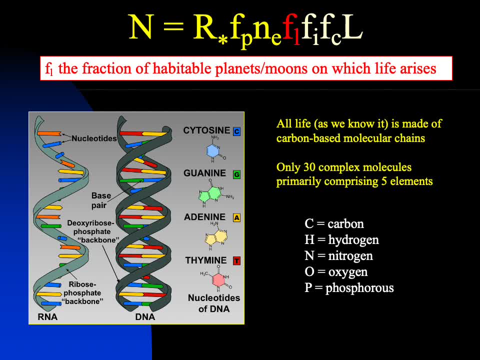 habitable planets coming into existence in the galaxy each year, And now that we know that rate- or at least we're trying to estimate that rate- we now want to step into the biology part of the astrobiology and start talking about the fraction of these habitable planets on which life actually 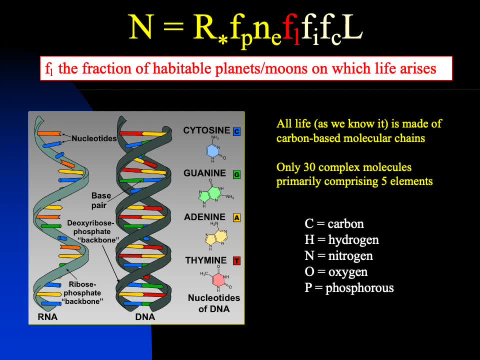 arises, And we mean any kind of life. We have not yet talked about civilizations or life forms that can form civilizations. We're not filtering for that yet, So let's talk about life Now. that's what this whole class is about. So we've discussed this before and I guess I really don't need to go. 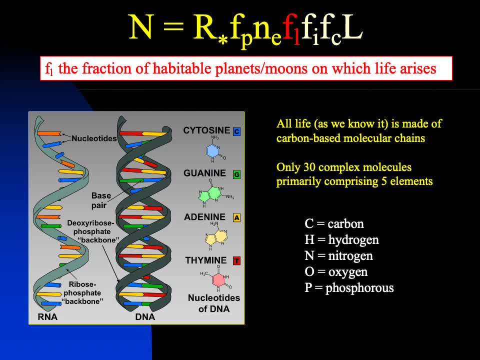 into a lot of details, but I just want to do some quick review to motivate why we might be optimistic about this number or this fraction, I should say this fraction between zero and one. First of all, as we've studied DNA and we've studied organic molecules, we've discussed the 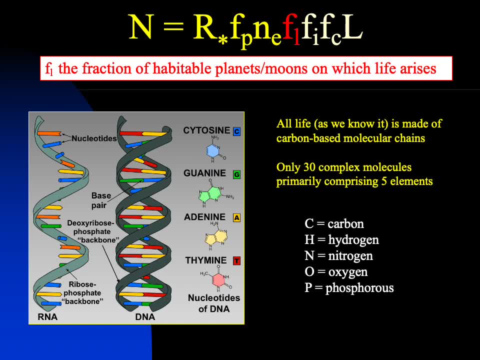 fact that all life, as we know it, is made out of these carbon-based molecular chains and that there's only about 30 of these complex molecules that are really engaged in life and metabolism. The interesting thing is that there's only five elements, which really are the primary elements that go into 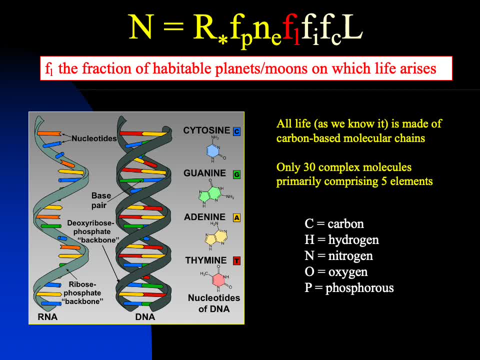 life. So you can think of chemistry and biochemistry as sort of the rules of language, if you will, And you can think of the molecules, the thirty complex molecules, as being the words that are constructed out of the letters, which are the five elements. so you have sort of 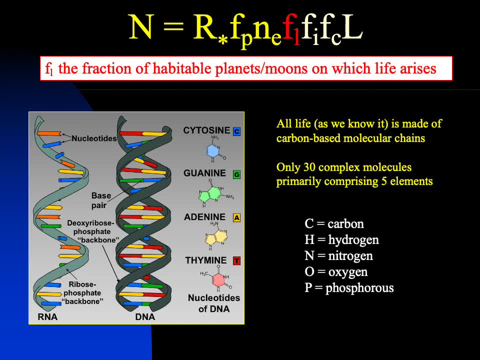 an alphabet of five elements which you from which you make words, which are the molecules- uh, about 30 of them- that that can be made, that are necessary for life, and then those molecules can come together following the laws of um chemistry, which is, like you know, making a. 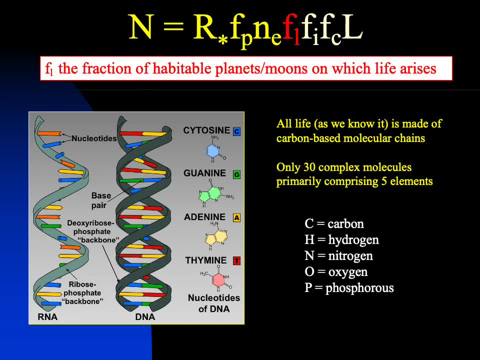 language- out of those um molecules, and so it's an interesting analogy. it kind of works in a way. and then if you look at the diagram on the left and you see the rna and the dna, i remind you that the, the backbones of those, are made out of phosphates, which 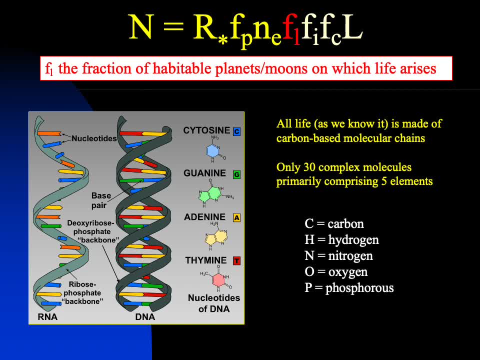 says a phosphorus, with three oxygens bonded to it and, other than that, the nucleotides of dna which are shown there: cytosine, guanine, adenine and thymine. if you look at those molecules, you'll see what are they made out of: hydrogen, nitrogen and oxygen. okay, so those are. and carbon, sorry. 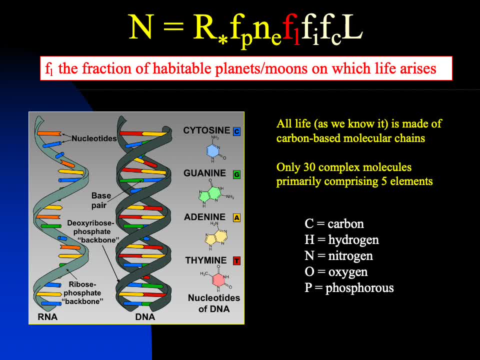 the carbons are not absolutely actually showed at each of the vertices of those molecules. so, except those, all those molecules, carbon, hydrogen, nitrogen, oxygen and then some phosphors, of course, that's uh for the phosphates which are involved with the atp, adp energy cycle and then also as backbone. 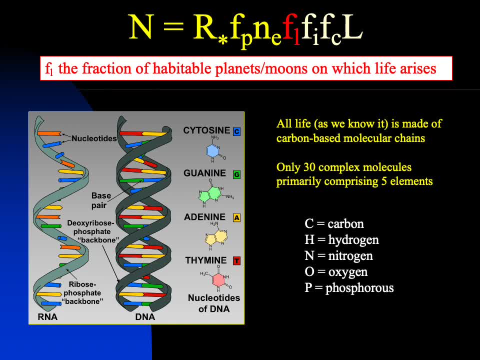 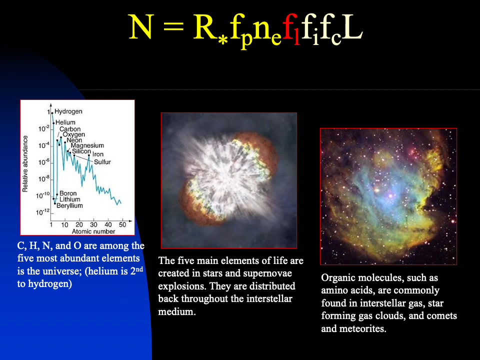 uh structure for your dna, and so this is the the basic uh thing about life is that it really boils down to five, mostly five, elements on the periodic table comprising these 30 molecules that then obey the laws of chemistry. so i will remind you that carbon hydrogen, nitrogen oxygen are amongst the five most abundant elements in the universe. 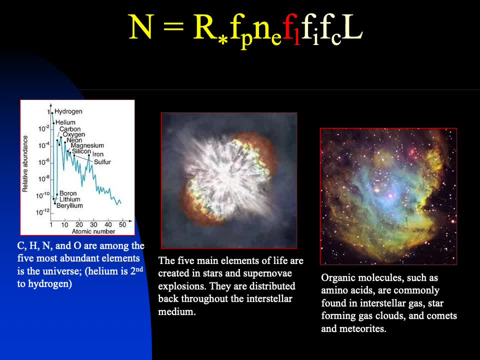 helium is the second most abundant, next to hydrogen. the helium is a noble gas and it doesn't really engage in biology. so on the left there is a little chart of the relative abundances by atomic number, which is basically: one is hydrogen, two is helium, etc. six is carbon, seven: 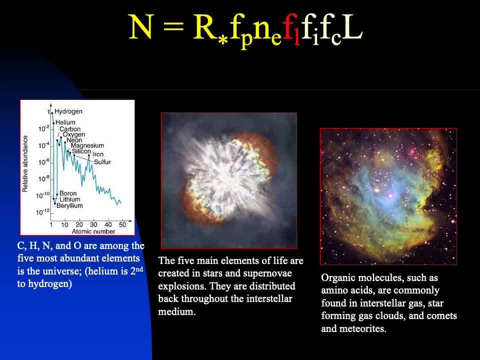 is nitrogen and eight is oxygen, and you can see that, uh, at the very left. you see the hydrogen and helium are at the peak, at the top of that abundance chart and as you go through a small dip, through beryllium, lithium and boron, you come. 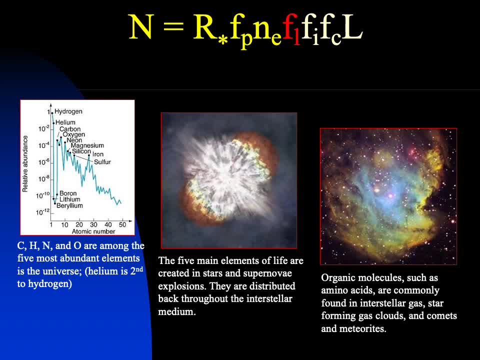 back up, uh, to carbon, and then, following carbon, it goes down a tad to nitrogen, and then back up and oxygen is even a little bit more abundant than carbon, and then, of course, it drops down dramatically with as you go up the periodic table. the point is that carbon, oxygen, nitrogen, 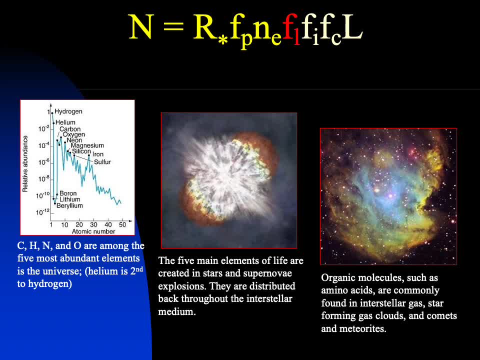 are in this particular diagram are amongst the top three uh elements that are forged inside of stars, and we remind you that hydrogen was forged at the time of the big bang about 13.6 billion years ago, so those are very old atoms, but carbon, nitrogen, oxygen that are in your bodies. 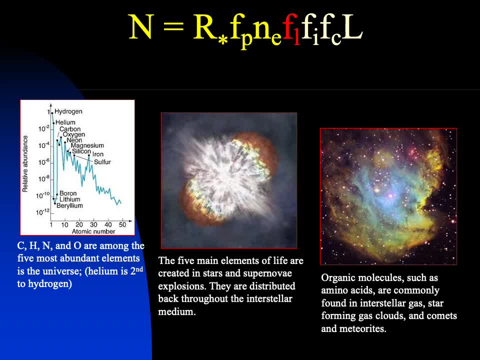 are more in the order of only a few billion years old to hundreds of millions of years old. um, it's the middle diagram is reminding you again that these elements are formed in the cores of stars- stars during their lifetime- That's what keeps them shining- is the nuclear fusion which creates. 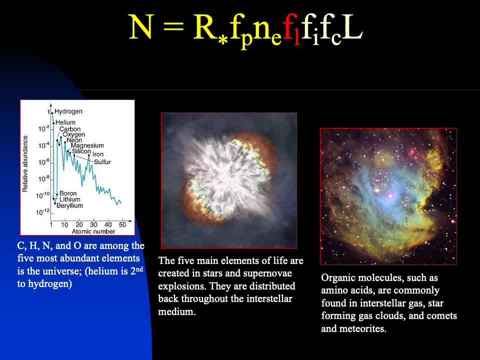 the heavier elements out of the hydrogen and helium that the stars first form from, And then the stars will age and they will explode. Some of them will explode: the high mass stars, things that are like maybe eight to 10 times more massive than our sun. Those kinds of stars will blow up. 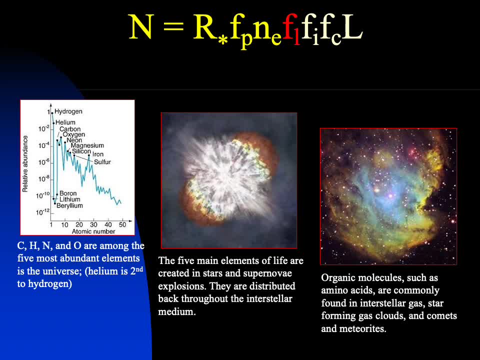 When they do, they blow their brains out, They blow all their chemical elements out into the gas between the stars, And this is how the carbon and the nitrogen oxygen are forged, and then how they are redistributed, so that you could form new solar systems and new stars with these. now more. 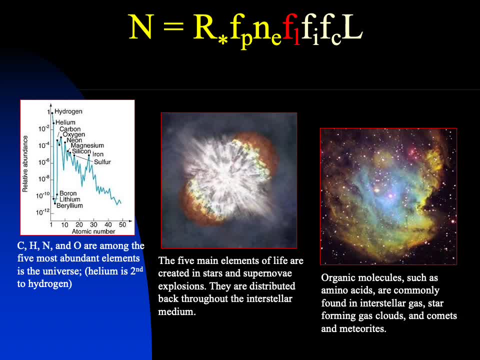 chemically enriched gas clouds. And then we see on the right panel there that organic molecules such as amino acids are commonly found in interstellar gas. They certainly are found in those stargates. They are found in those stargates. They are found in those stargates. 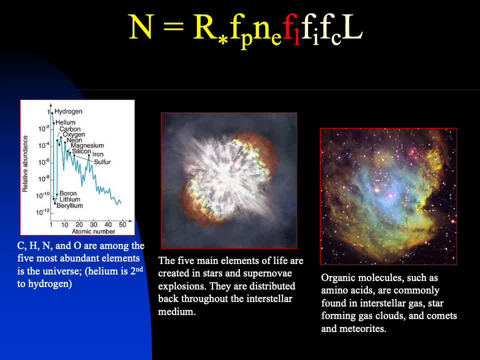 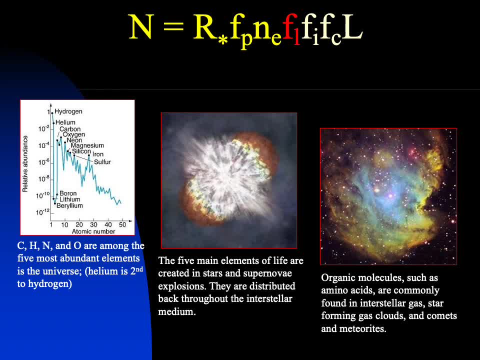 with organic compounds as well. So organic compounds are naturally formed chemically. They're naturally formed out of those five basic elements which are forged in the cores of stars, And again, they are the five most abundant elements in the universe. All of that bodes. 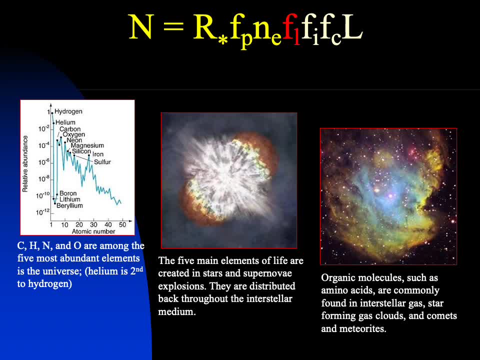 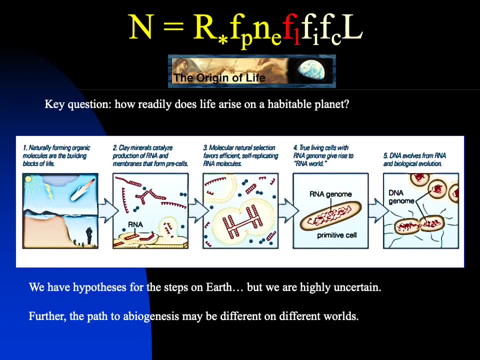 well for the universe, really creating the ingredients for life. The real question, of course, then becomes: how does life actually arise? from gas clouds that coalesce, that have carbon, nitrogen, oxygen and hydrogen and phosphorus and them, And of course you get concentrated on a planet. But how easy is that process of going? 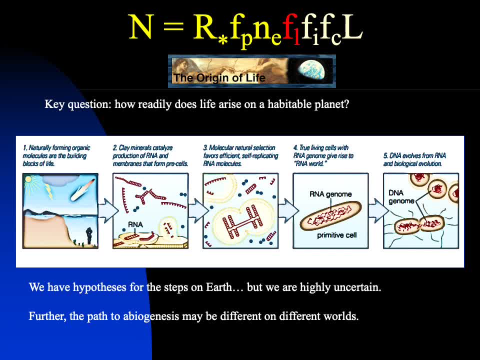 from biochemistry, or I should say organic chemistry, from organic compounds with chemistry, to reproductive biochemistry, And so we had a whole chapter, a whole module on this, And I remind you of the five steps We discussed for our hypothesis, for the steps that may have taken place on the planet Earth. 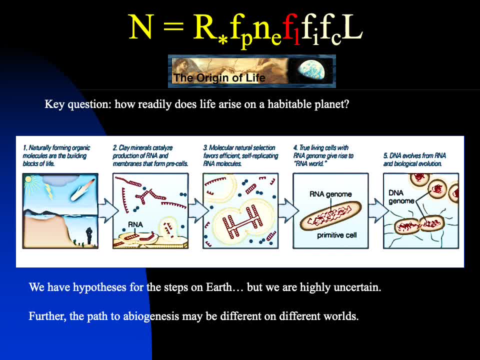 And so basically number one: if you put together these compounds in concentrated areas and you have energy for them, you might get something called an RNA world, where the RNA is using something like clay to help concentrate it and then catalyze the duplication of mirror versions. 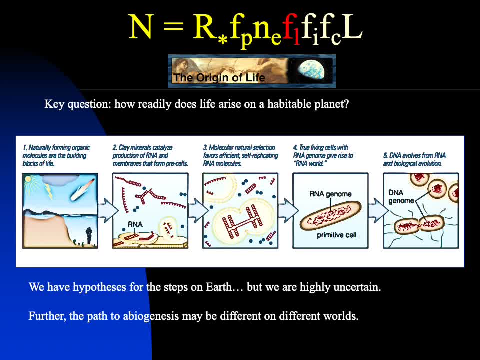 of the RNA. We talked about lipids and amino acid bubbles. that then might encase some of the RNA. That's step three. and then which you might actually have a competitive process- I shouldn't say competitive, but one of which: those which are RNA which are duplicating in the bubbles. 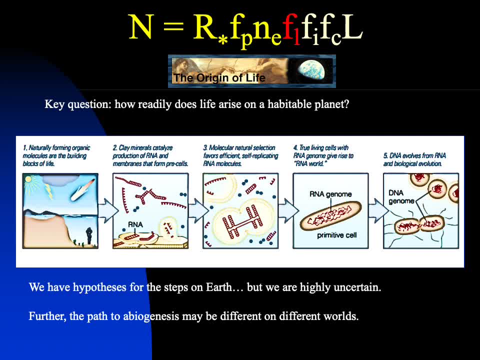 might be more well-protective And therefore this becomes the more commonly present form of this reproduction, as kind of an unequal reproductive success argument from Darwinism And then of course, somehow going on from the prokaryotic cells developing into prokaryotic cells. 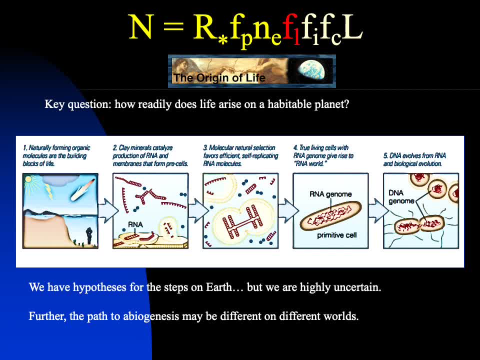 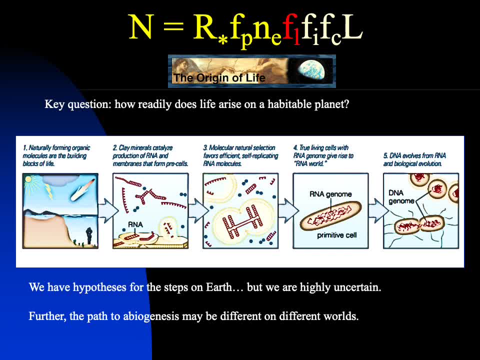 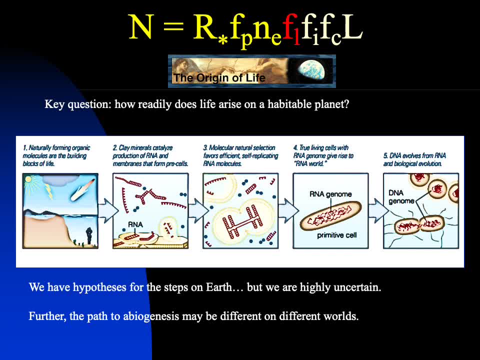 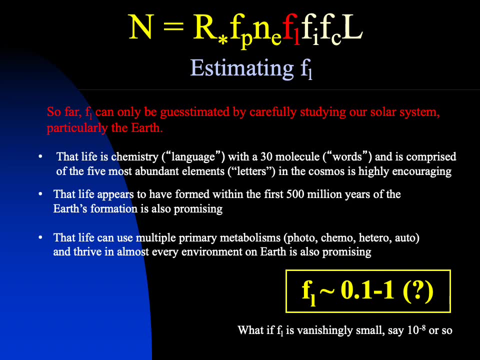 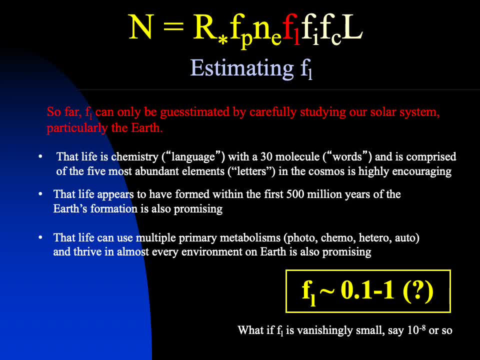 And then, of course, what we can do is we can use the JWST, the Webb Telescope, the TES and WFIRST to try and measure the atmospheres of these exoplanets. And then we briefly talked about it in a previous lecture- where NASA had pointed the Galileo Telescope at Earth, Venus and Mars and measured their atmospheres and looked at the chemical composition and showed that you could definitely tell that there was water vapor and ozone on the Earth which was not present in the atmospheres of Mars and Venus. 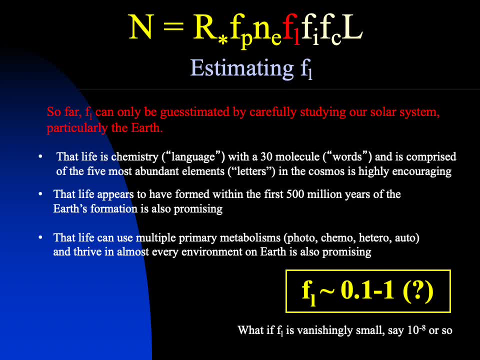 And we also watched a space time video Which talked about how out of equilibrium methane is and the chemistry of the atmosphere is that would suggest that there's life. So if we can use the TES, the TES, the TES Telescope and JWST and WFIRST to measure these out of equilibrium conditions in some exoplanet atmospheres, then we may be able to say, hey, we found biomarkers. So if we can use the TES, the TES Telescope, and JWST and WFIRST to measure these out of equilibrium conditions in some exoplanet atmospheres, then we may be able to say, hey, we found biomarkers. So if we can use the TES, the TES Telescope, and JWST and WFIRST to measure these out of equilibrium conditions in some exoplanet atmospheres, then we may be able to say, hey, we found biomarkers. 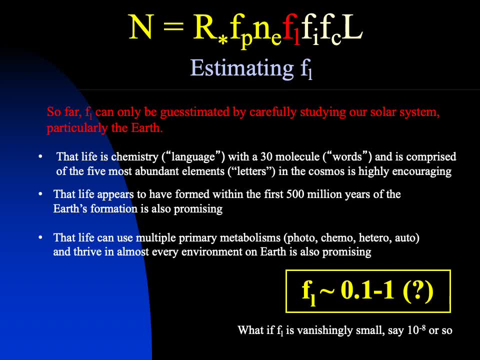 It's important to get a sense for life on some of these other exoplanets. Again, 20 years, come back and talk to me and we will probably have a much better sense of F sub L And in a sense I guess I said before that RSAR, F sub P and N sub E were really the only astronomical type of variables in the equation. 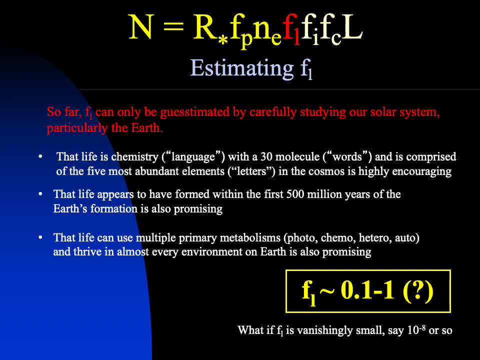 But now I'm realizing that astronomy is probably going to help us learn f sub l as well. um, that's interesting something to think about. so, um, let's review the bullet points here. um, life is chemistry, biochemistry. that's the language of about 30. 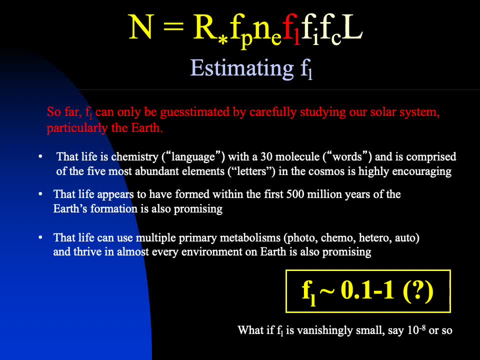 molecules, which are the words that form the language, and it's comprised of the five most abundant elements, which would be the letters that make up the words um, in this cosmic, in the cosmos, and the fact that this is uh, such a simple and small number, uh game, and they're the most abundant. 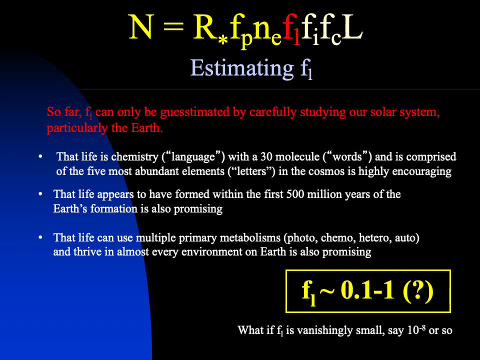 is really encouraging. now, if we look at the history of the earth, which we talked about in a previous lecture, we found that the evidence that life formed within the first 500 million years is also very promising, and we saw that ancient stromatolites um that formed from bacteria. 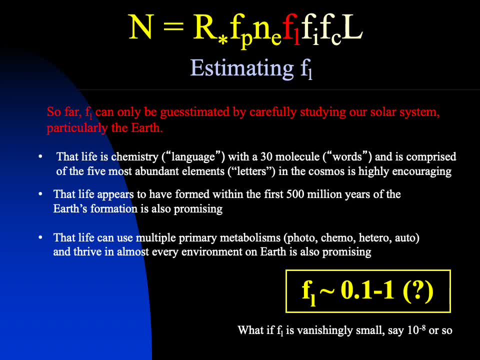 colonies that were present as early as 3.5 billion years ago, so that that's very encouraging that, um, that life took hold, the simple life took hold on earth very rapidly. um, and then the fact that life is very robust under a lot of various conditions, and 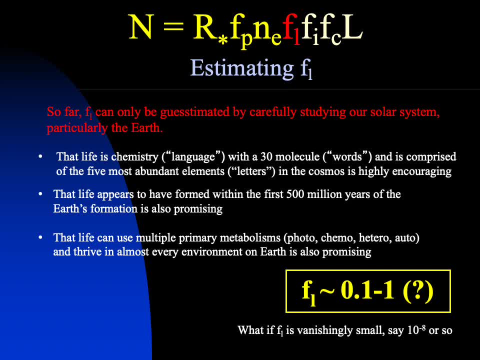 environments on the earth, from very cold uh dark places to very hot places- what we would call the extremophiles- and that there are different versions of primary uh metallurgy that are present in the universe, and that's why we're talking about the first four metabolisms, like the: 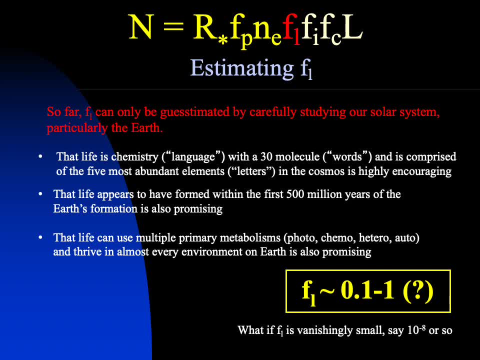 photo heterotrophs and the chemo heterotrophs and the photo autotrophs and the chemo autotrophs, and if you remember those four metabolisms, so that you don't always have to have life be photosynthetic, uh or um, or that actually it can just use chemicals as its energy source, um, even. 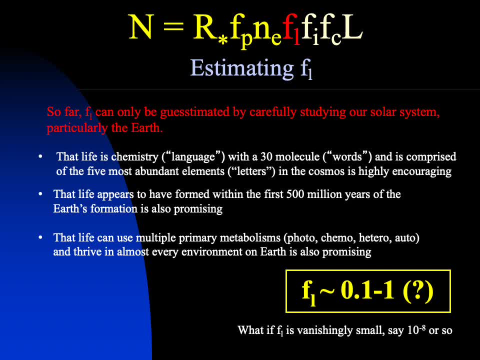 in dark areas or very, very hot areas. that would be hostile to life. um, like ourselves, you know humans okay. so the fact that there's this, that every ecological nesh of the earth has basically been exploited by this thing called life, is also very promising. so we have a little box in the corner and it basically is: f sub l equals point one to one. 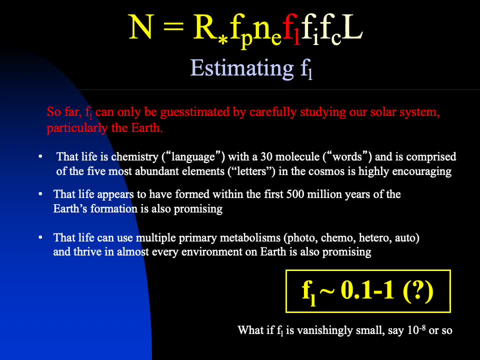 question mark. okay, so if earth is typical, if earth is typical and common, well, it doesn't matter if, if, if you have a habitable planet like earth, uh, and earth is typical, then we would be very optimistic that f sub l should be close to one now. um, maybe in our solar system we find that. 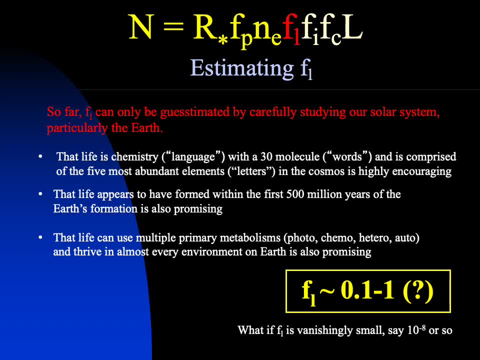 when you consider the moons that are habitable and the fact that mars was habitable for a while and then not habitable, and and and whatnot, maybe we would be less optimistic and say, well, it's one out of ten, but even one out of ten is extremely optimistic in the overall scheme. 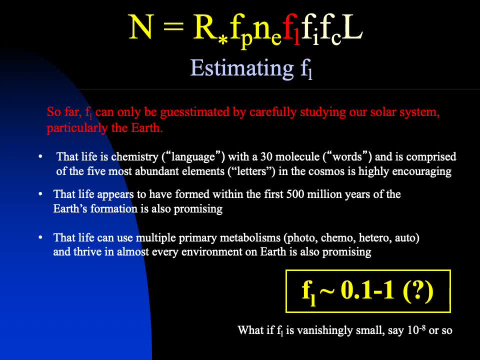 given how many stars there are and how many planetary systems there are out there in the galaxy. what we would be worried about is if, in scientific terms, what we call, we use the term vanishing, or if it vanishes, if f, sub l was to vanish- and that's a fancy way of saying if it. was to get very close to zero or to go up and down and to move, continue to go down. if the thing South, Western data is to days, if we want our Earth to just be very close to zero or to go up and down and suddenly need more information to texture the current structure to, we could just be out of an 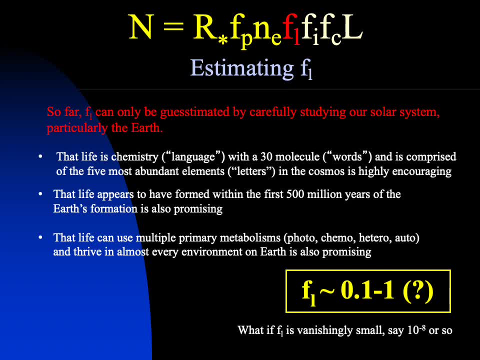 to zero, So vanishingly small. say 10 to the minus eight, which is, you know, 0.000080 is with a one, And that would be one out of a hundred million. So that really now is a small number, That's. 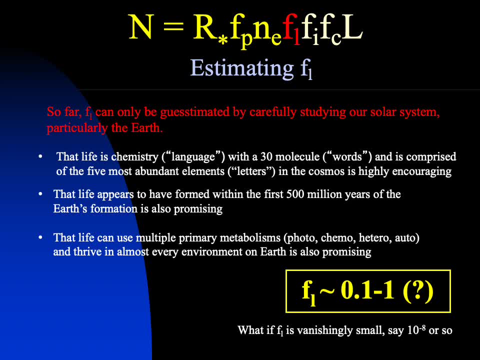 you know, it's not zero. F's and L's number between zero and one, It's not zero, but it's vanishingly small. And so once you, as you know, when you multiply a string of numbers together- which is what the Drake equation is- you're multiplying a bunch of numbers together. 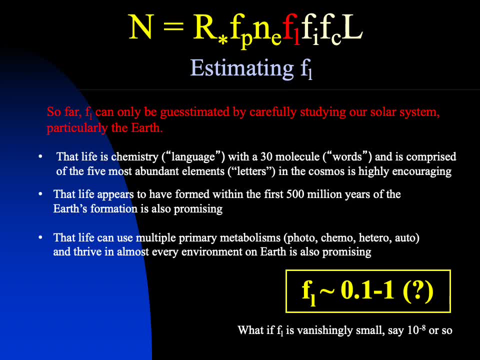 If any of them is zero and you multiply anything by zero, you get zero back, And so clearly F's and L's can't be zero. because here we are and we're talking about F's and L's and we're living creatures, But is it vanishingly small? Because if you multiply these other 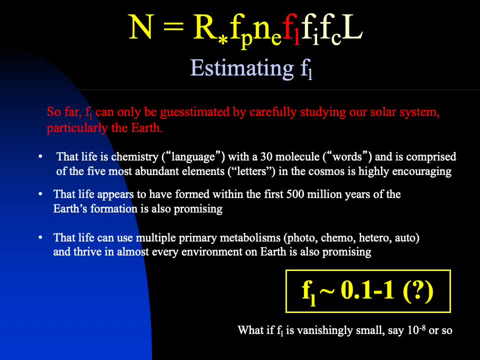